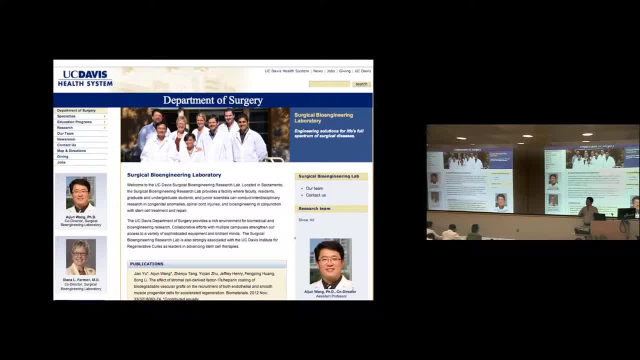 So the surgical bioengineering lab, as I said, is in Research 2, the third floor. We have quite a few faculty members there: Dr Farmer, myself and Dr Perez, Dr David Sahar and Dr Ian Brown are in the Research 2 building for research. 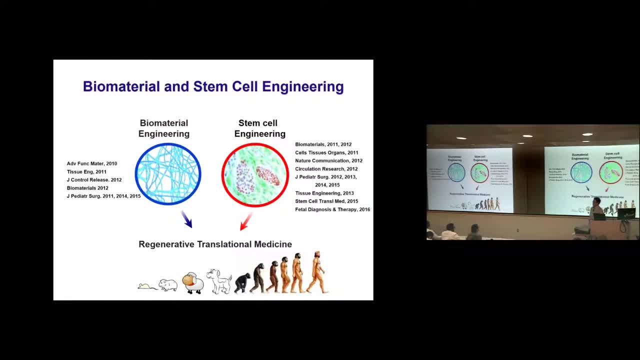 So for my own research interest, I was training bioengineering at UC Berkeley doing my postdoc. So my research interest, My research interest, is mainly focused on tissue regeneration by using bioengineering tools and technologies, especially stem cell engineering, to make some biological stem cell product or therapeutic and biodegradable polymer or extracellular matrix, scaffold-based biomaterial engineering. 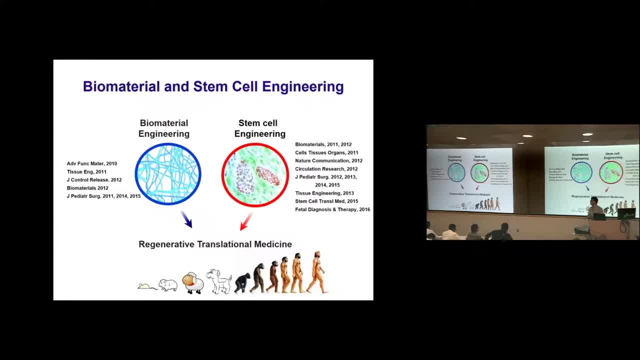 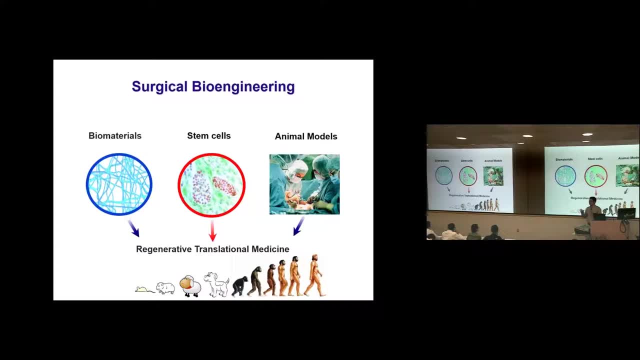 So the ultimate goal is to combine biomaterials and stem cells for different disease treatments. So currently in the lab we have basically three different arms for doing the different research projects. The first arm is biomaterial. So we're doing a lot of scaffolding, surface modification of devices, 3D structural fabrication for a scaffold, and I'm going to talk to you about that later. 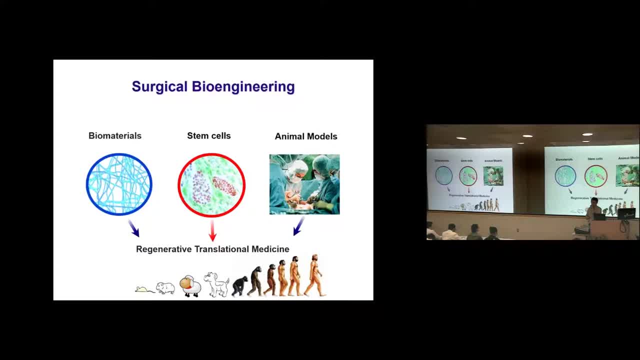 And stem cells actually is the main research focus in the whole lab, especially stem cells. So we have stem cells from different sources, so especially stem cells from induced pluripotent stem cells and stem cells from perinatal tissues, different tissues such as placenta or other perinatal tissues. 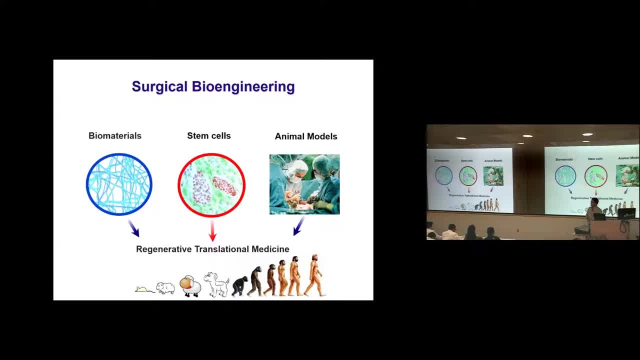 And we have a large arm of animal modeling for different human diseases, So I'm going to talk to you about that too. So we are focused on regenerative medicine, which meaning we want to regenerate tissue or tissue, We want to reduce the damage, we want to interrupt or you want to improve the center of care. 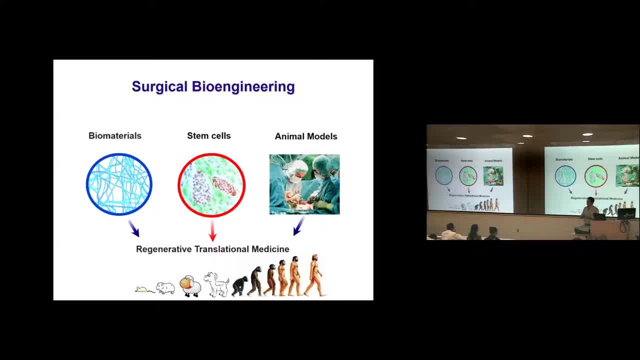 We're doing translational research. We're trying to build up some products down the line so that we can use it for a clinic. So hopefully today you will find something that's interesting to your practice or research interest so that you can always come to the lab and talk to me or other lab members and see what we can do for you. 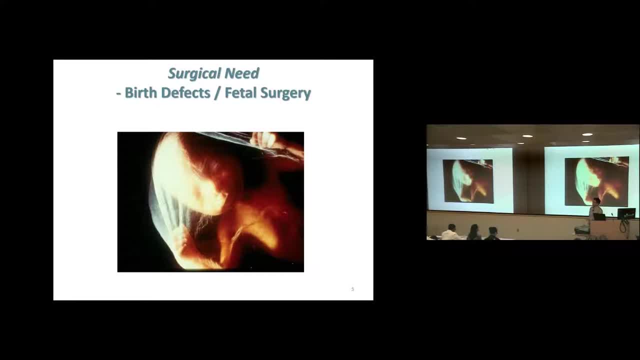 So a few examples of what we can do for surgical conditions. Surgical conditions: Surgical conditions Number one, that's our major research focus right now in the lab is some bioengineering approaches for birth defects or fetal surgery. So, as you may know, Doug Farmer and I are co-PIs on a large CIRM grant supporting our spina bifida research. 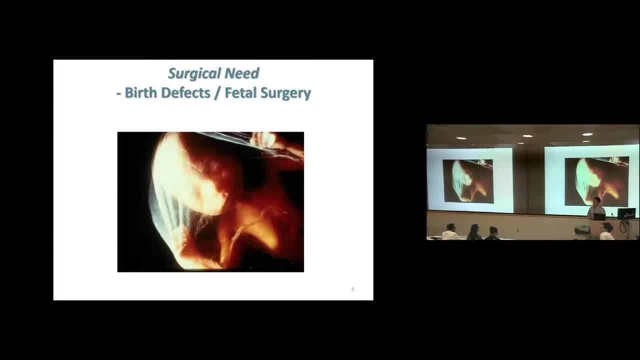 I believe most of you have seen the video, but I'm going to show you that again today. So just to show you what we can do by combining surgery with bioengineering. So just to show you what we can do by combining surgery with bioengineering. 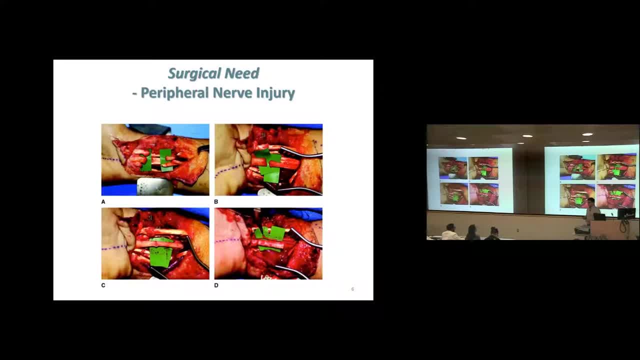 And how we can do things differently. So, for example, other applications. So for example other applications like proof of nerve regeneration or peripheral nerve injury, And you want to, especially for large defect, large gap, that you cannot directly suture them together. 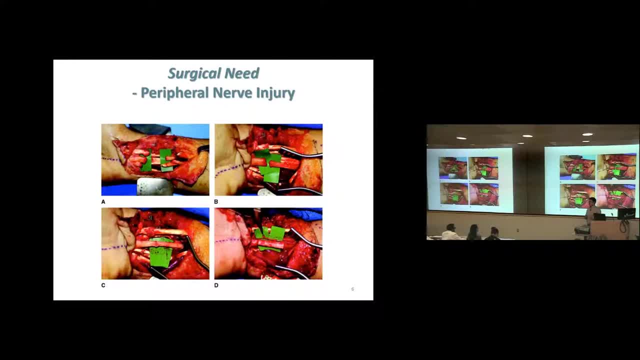 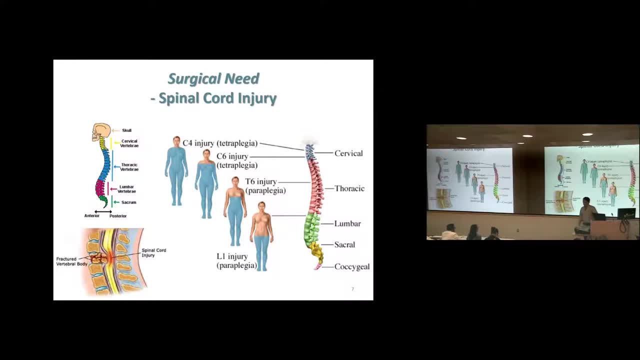 how you can use some devices to help the tissue regeneration. And the third one was just a like a very commonly seen spinal cord injury, for example. So when the spinal cord tissue, So the spinocord tissue, is damaged, it's really very difficult to regenerate. so when the spinal cord tissue to regenerate. So what we can do in the last quarter is that we canGER JE olivine and講 ش the suffered-orền to regenerate the spina bifida and people with putting Deutsche sevi Majda, an antudiagnostic preserved poinsettia. 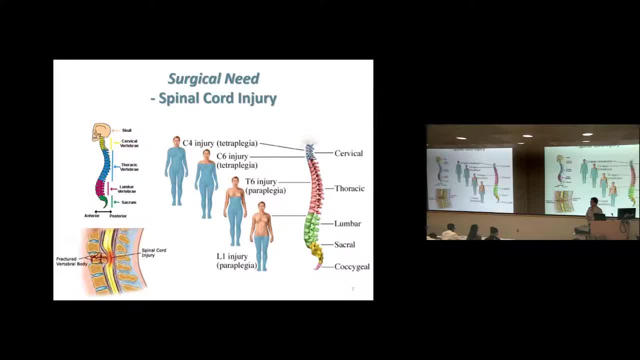 in the lab is to add some biological components or some biological tools to help the body to regenerate better the core tissue or to protect neurons from further damage- Something like that. I'm going to talk to you about the stem cell related products in a little bit. 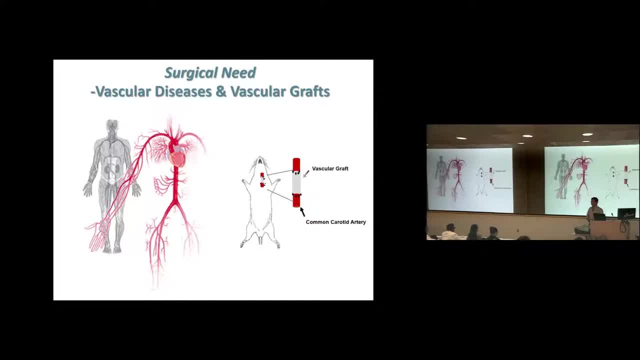 And also cardiovascular diseases. for example or so for blood vessel regeneration or bypass blood vessel, Can we use bioengineering approaches to make a better bypass product that tissue can like, especially endothelial tissue. endothelialization can happen faster or better to cover the surface. 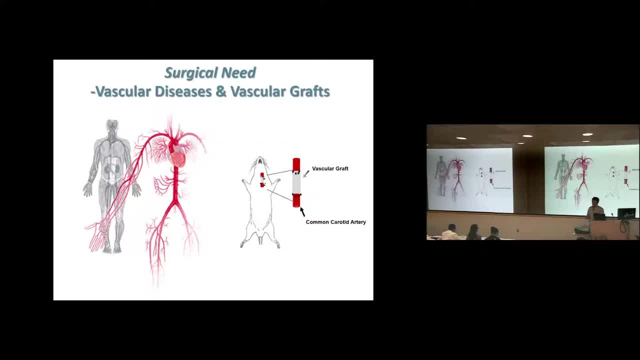 that blood is contacting, So that once the endothelial cell is covered on the surface, like sooner than the thrombosis or other bad effects happening, the patency will be improved. So these are just a few examples, But we can do a lot. 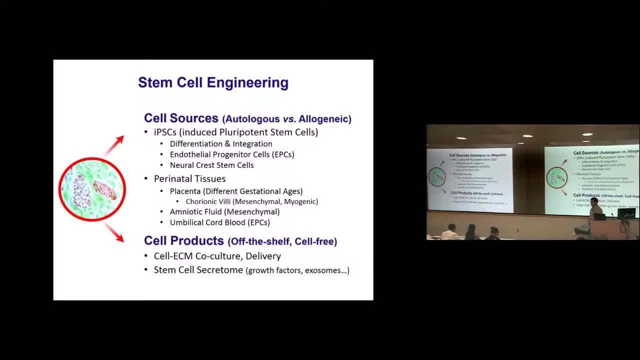 We can do a lot of other things too. I'm just trying to stop here for a little bit and think about what's your research interest and what the bioengineering tools and technology I mean. I can only cover very little bit today. 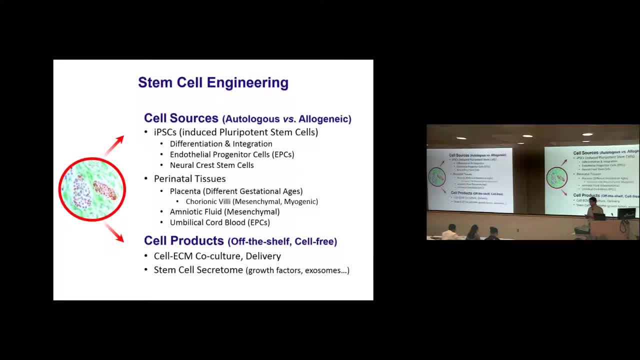 But there are so many things happening in the engineering world, and bioengineering especially So, like cell expansion, culture, all those things, And you know: devices fabrication, 3D printing, surface modification, just to make your device more personalized or more your disease-specific or your application-specific more effective. 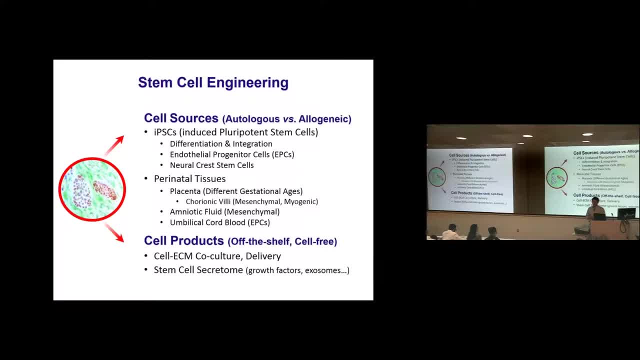 And also some devices, for example bioreactors and device fabricating capability, and also a lot of animal modeling for your specific research interests. I think we can probably help. So let me start from stem cell part. So, as I mentioned, I mentioned earlier 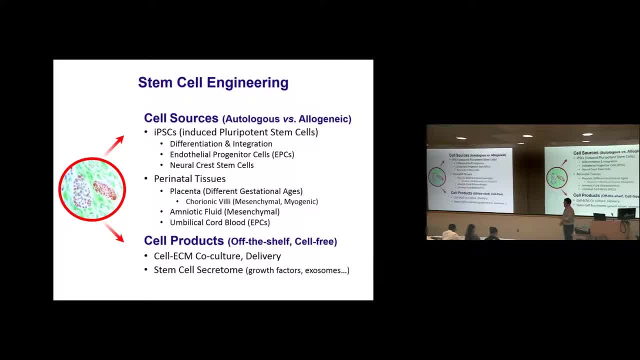 So we have many different sources of stem cells. Today, I'm going to talk to you about two main cell sources that we can use for research and for future applications. Number one is a. well, as you all know, the autologous cells might be the best cells for. 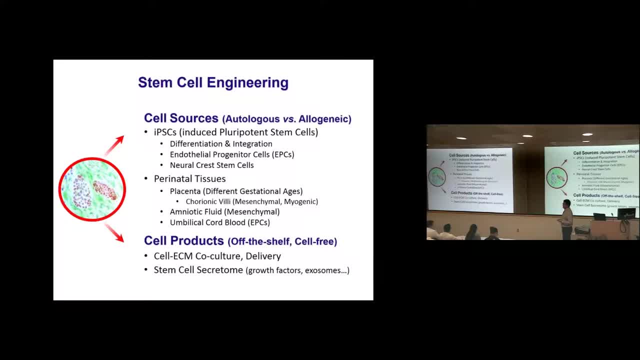 the patient-specific applications. So how can you get autologous cells for different type of cells? If you think about this for a minute, it's not easy, right? For example, if you want to get some endothelial cells from a patient. 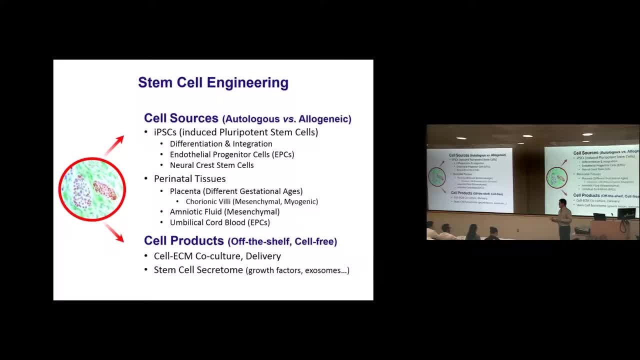 It's not easy to get endothelial cells. You have to cut probably a segment of a blood vessel or somewhere that you can sacrifice to get tissue and cell isolation. those kind of process very difficult. But there's a new technology called reprogramming which is, I believe, most of you would know. 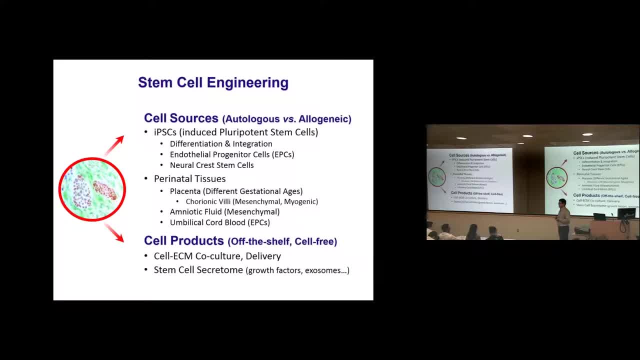 IPS technology induced pluripotent stem cells, which is to induce patient fibroblasts, for example. These are biopsy cells that you can use the antiviral system or other transduction system to make these fully differentiated cells into an embryonic-like cell stage, and then you 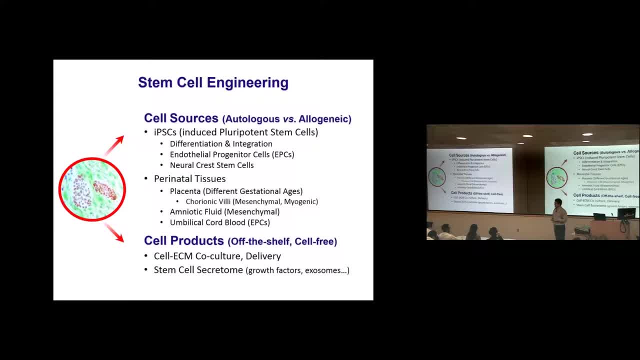 can differentiate those cells into the cell type that you want, Any cell type, basically All the cell types that you can see in the body. So today I'm going to talk to you a little bit about some research that we're doing on here which shows the promise for making patients. 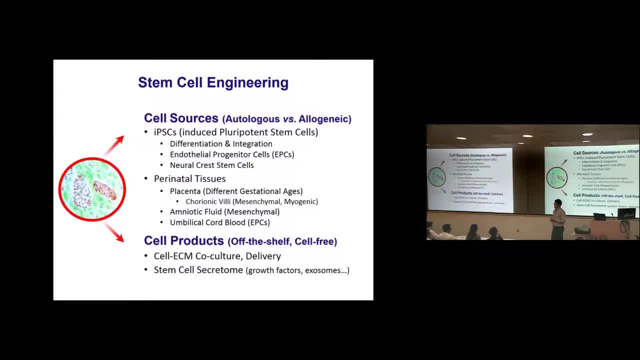 Okay, So we're making patient-specific cells, different cell types for any specific disease treatment, For example endothelial progenitor cells that we can differentiate from human iPS cells. So human iPS cells can be generated from any skin biopsy urinary sample, many, many fully. 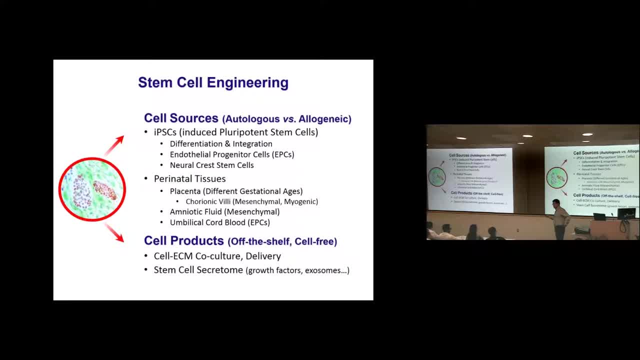 differentiated cells. That's very well-established- It's a 2012 Nobel Prize science actually. It's very well-established now in the lab- And neural crest stem cells That we have been working on for quite a few years. So it's another type of multipotent stem cells that can differentiate into multiple lineages. 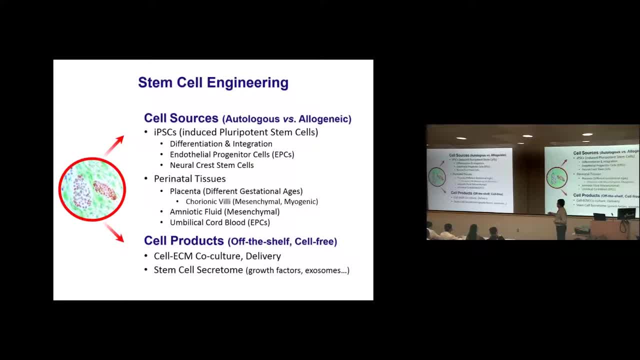 So you can use that for different tissue regeneration purposes. So another portion is perinatal tissue, especially for our birth defects or congenital diseases. So from perinatal tissues, placentas especially. I'm going to talk to you about that, how you 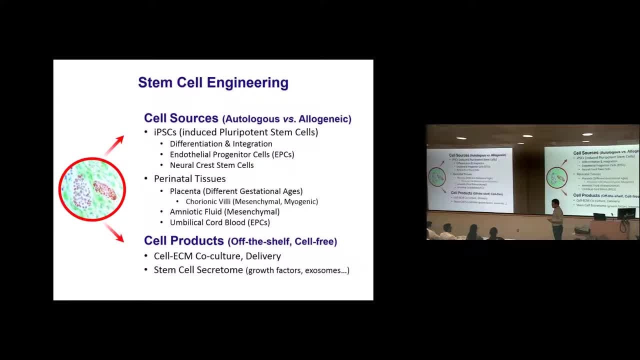 can generate stem cells from- excuse me, Okay, From- placenta at different gestational stages, And also there are some other tissues available for cell derivation, for example amniotic fluid samples. I'm going to talk to you about that too. 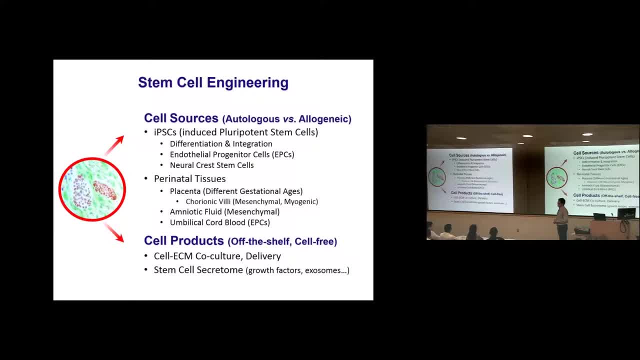 So another one is very well-established in the lab as well- is umbilical cord blood sample. So if you get some umbilical cord you can get the blood sample. You can generate a lot of very young and very immature progenitor stem cells, for example. 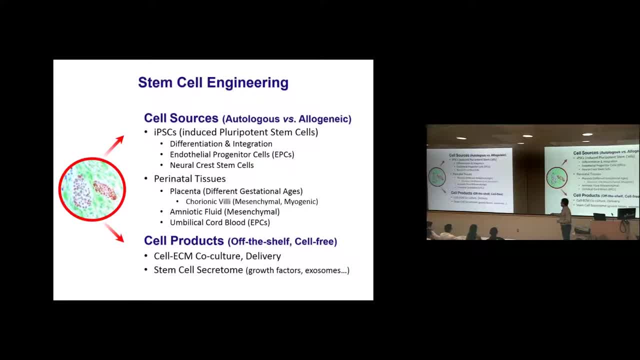 endothelial progenitor cells So you can use that for your different applications. So, based on all the stem cell or cell research, we are trying to establish some stem cell or cell product. So either a cell product that you can use off the shelf or you can process the cells. 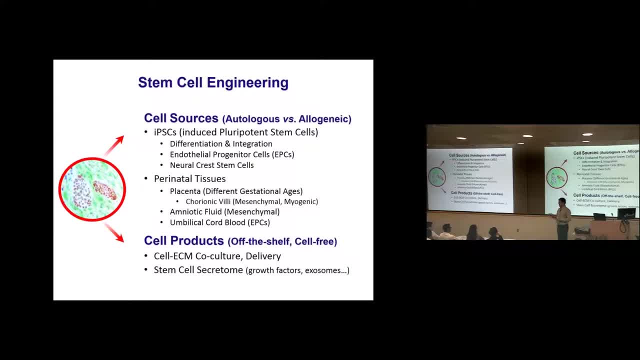 with some ECM or scaffold, So for different applications you can ship to some other places. That's the hope for cell product development. On the other side we can develop some cell-derived products. Okay, So not live cell product, it's a cell-derived product. 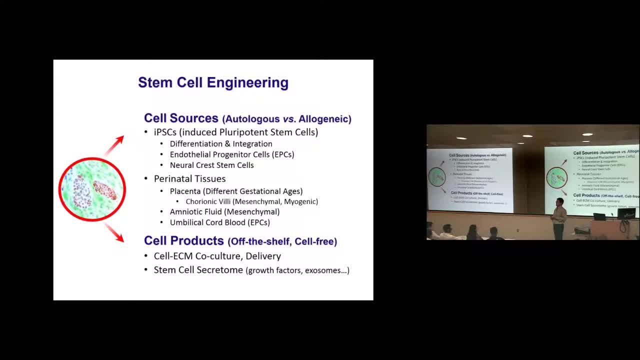 For example, cell-secreted stuff in the culture, media that we can isolate or concentrate- So condition media, for example, or exosomes- So I'm going to talk to you about that in a little bit as well- like growth factors or exosomes that are produced by cell culture. 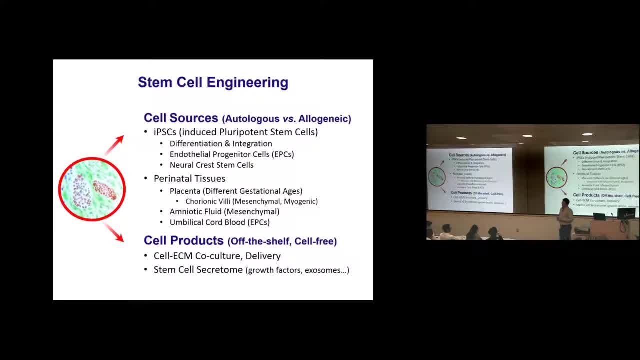 So you can culture a lot of cells in vitro, expand many, many flasks and then you collect the cell condition media And then you extract or purify the components that you want to have for specific applications. So first I'm going to talk to you very briefly about the differentiation of human-derived 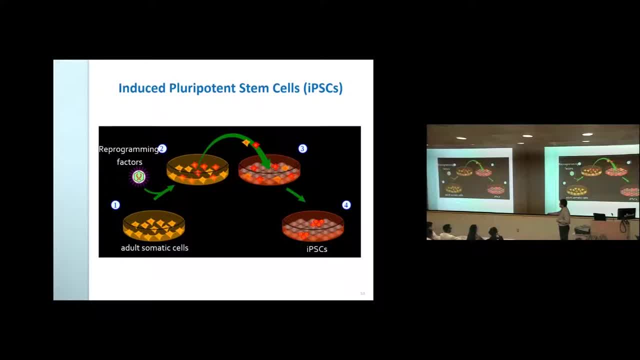 iPS cells into the cell type that you want to use. So, as I mentioned, this is the process for reprogramming. It's very simple, very straightforward. You have some adult somatic cells You can easily get from patient biopsy- skin biopsy, for example- and then culture these. 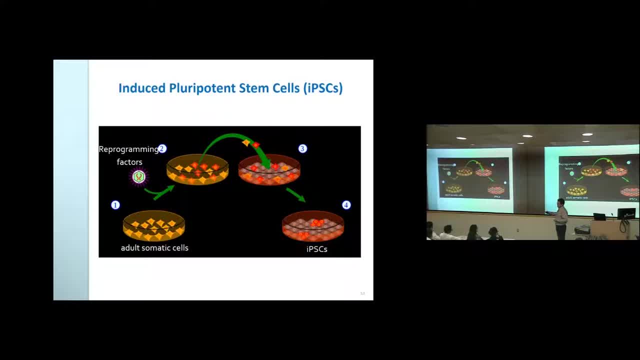 cells from the skin biopsy, Okay, Okay, So in the case of a biopsy sample, you can reprogram these cells. There are so many different ways nowadays to reprogram cells into iPS cells, like embryonic stem cell-like stage, so that are pluripotent, meaning they can differentiate into all the. 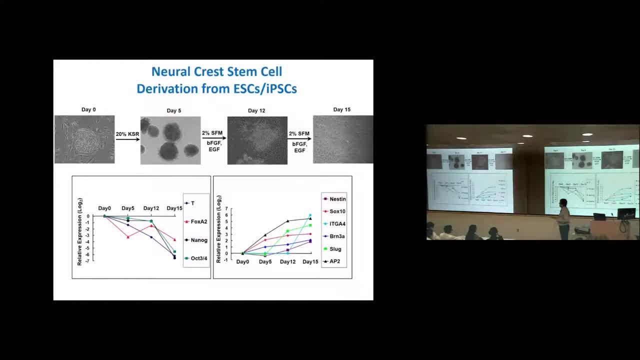 cell types, all the lineages in the body. One direction that we can go is to use pluripotent stem cells to differentiate them into neural crest stem cells. So why would not be? Why would it be optimal to use iPS cells directly for therapy? 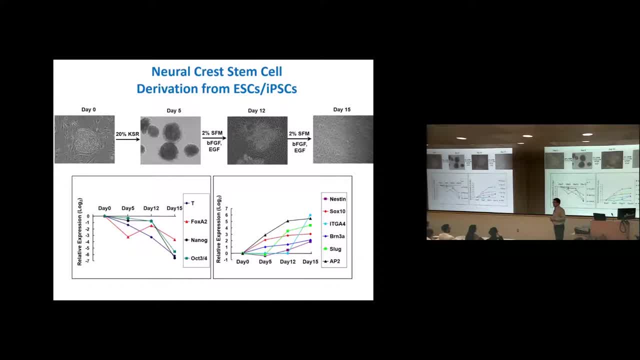 If you think about this for a little bit, because these cells are pluripotent, they are very. They can form teratoma very easily. They're growing very fast and if you transplant these cells directly into an animal model, for example, so they will develop teratoma very fast. 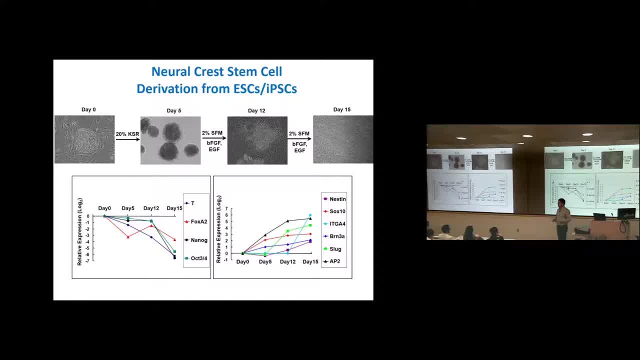 And they are fast proliferating. they're also making all different type of tissues that you cannot basically control them very well. But once you differentiate these cells into certain stem cell- instead of pluripotent, maybe multipotent or unipotent- progenitor cell stem cell lineage, that means they can. 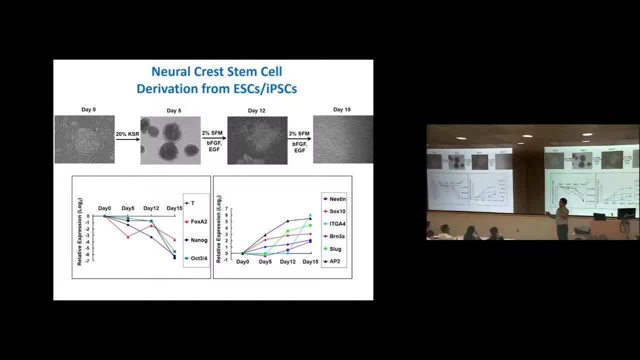 only go to certain pathways instead of going into many other different pathways. So that way you can control the cell fate, basically to a range of the differentiation potential. So this is one example. Neurocrest is a very important developmental, transient developmental stage. 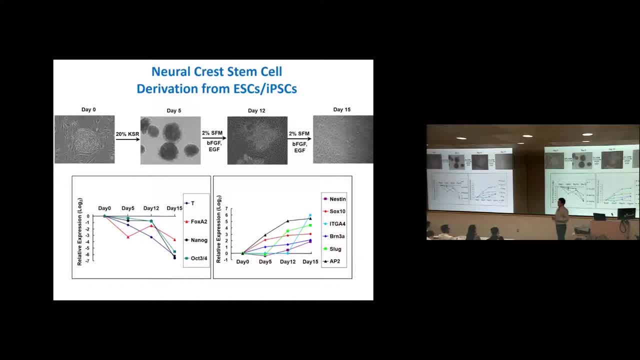 So it's very difficult to get neurocrest cells from the embryo. You have to destroy embryo at certain developmental stage to get those cells. And they are multipotent. They can make ectoderm tissues and they can also make mesoderm tissues. 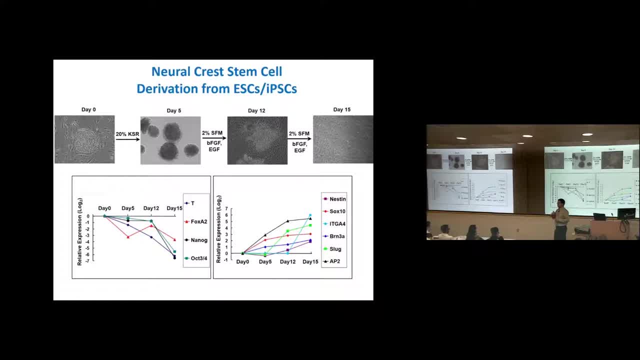 So they are multipotent. They are very important for making a lot of the tissue in the adult stage But it's very difficult to get them from From development. But using iPS technology you can establish a differentiation protocol that can control the iPS cells to go into neurocrest stem cell stage very specifically. 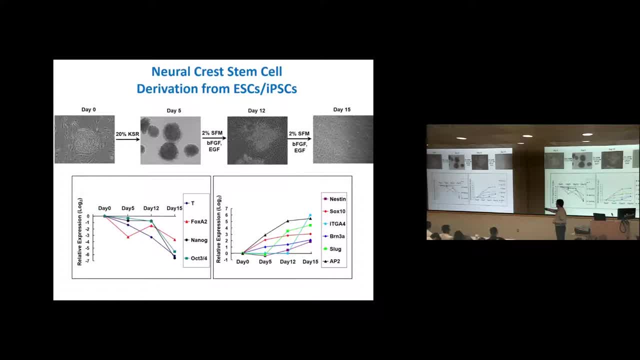 For example, here we have identified a protocol that you go from iPS cells through different stages and then you get monolayer. So iPS cells like embryonic stem cells, they are cultured in clones, So they can see very well-defined clones. 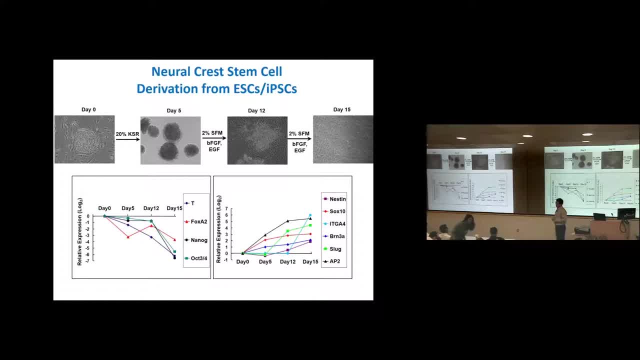 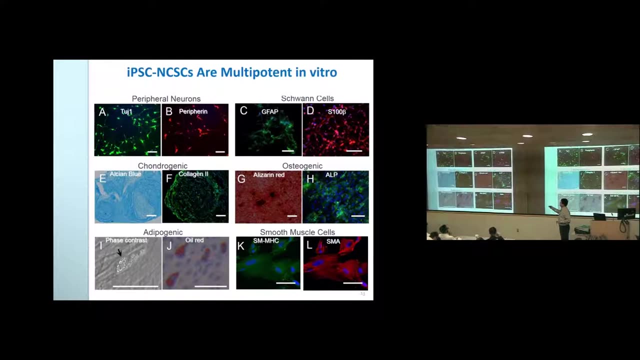 But once they differentiate into certain multipotency, multipotent stage, they will Like for neurocrest stem cells. they're monolayer culture, They're not making any teratoma in the B-vivo applications And we also show these cells differentiate from iPS cells. 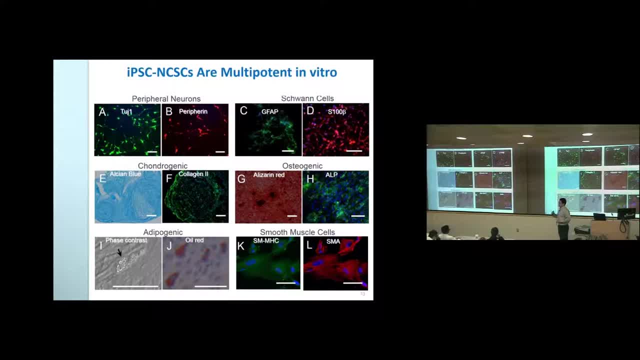 They're multipotent, just like embryonic neurocrest stem cells. They can make neurons, They can make strong cells, They can make all these mesodermal lineages, Chondrocytes, Osteoblasts, adipocytes, submarsal cells. 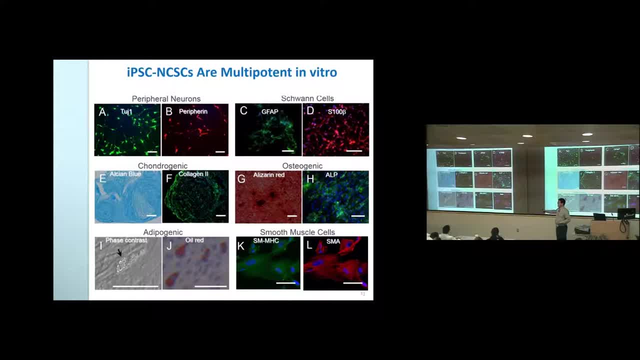 So if you stop here for a little bit, you can, So you can think about. You get the skin biopsy from a patient. Actually, you go through your reprogramming and differentiation. Now you get all different type of differentiation cell that you want to use for this patient. 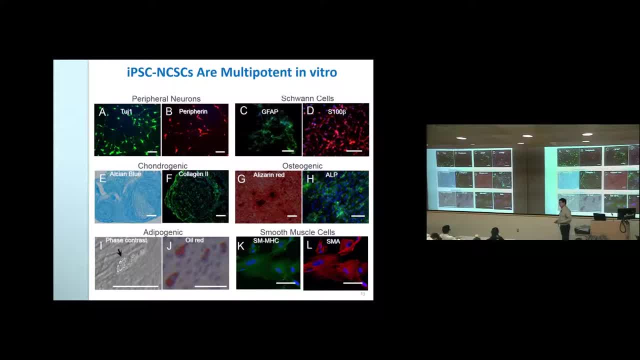 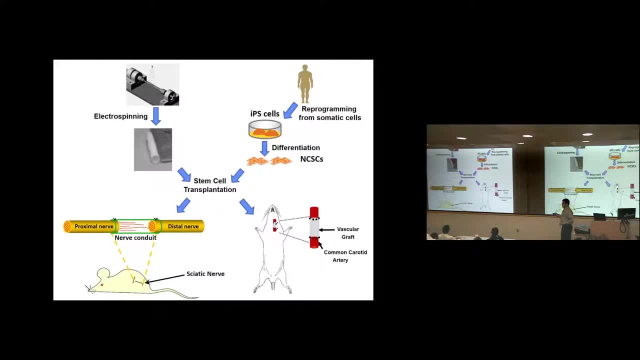 It's patient-specific, There's no rejection. There's no immune rejection, that Also there's allogeneic, like from another donor, for example. So there are many applications that we can use for Hi, Hi, Hi Hi. 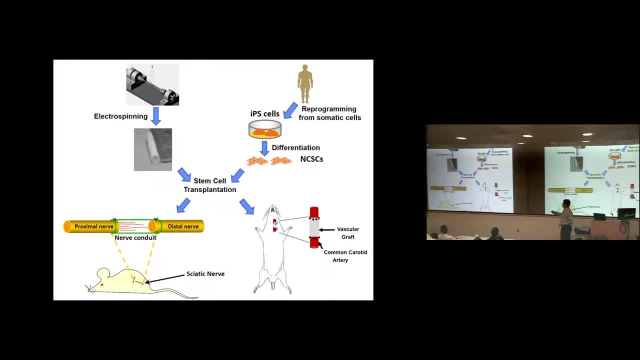 for the reprogrammed iPS cells and differentiated cell types, in combination with a lot of scaffold technology that I'm going to talk to you about in a little bit, So you can do stem cell transplantation for different disease treatment. So this is one of the diseases that we worked on. 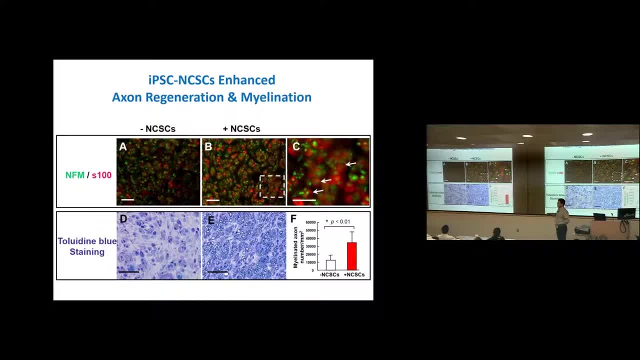 which is a peripheral nerve regeneration. So in the rat-selective nerve injury model we made a one-centimeter gap, which is a very long gap for a little rat. So, without anything, if you don't do anything, just leave the gap there. 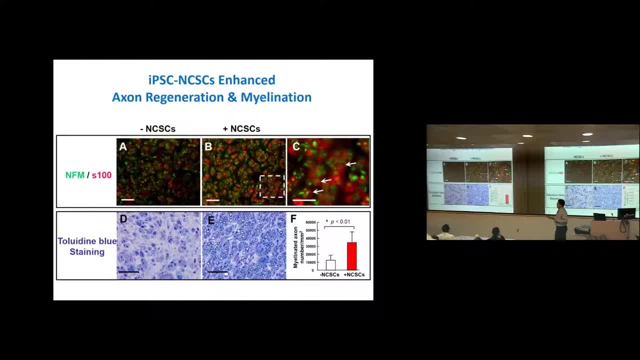 The rat cannot regenerate the nerve tissue, But with the bioengineered scaffold and stem cells actually we can see here, so you can see in both groups. you see in the middle of the nerve conduit, you see some tissue regeneration in the middle of the conduit. 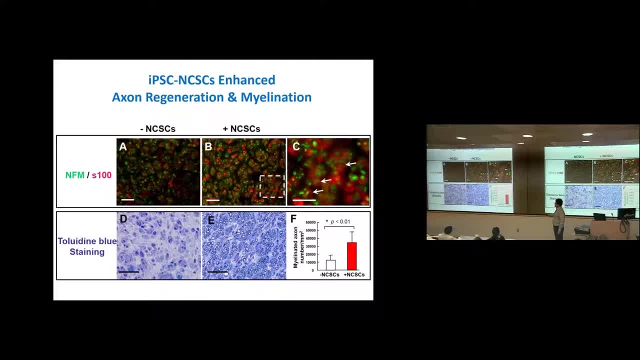 But with human stem cells, neurocrest stem cells, which is a Schwann cell precursor cell actually. so in the immune-deficient rat model you can see many more melanated axons which are contributed by these transplanted cells. 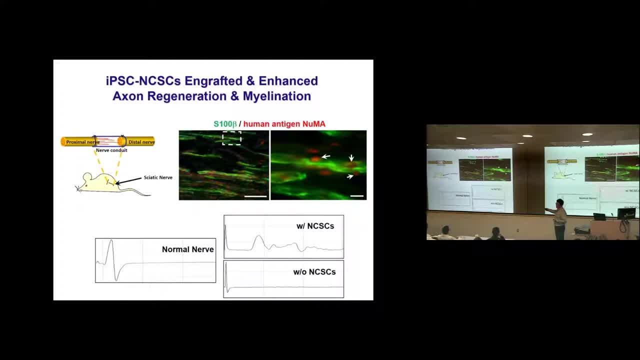 as you can see here. So the green is S500 beta, which is a Schwann cell marker And human antigens. shown here in nucleus is a human pneuma, which means in the cross-section, or this is actually longitudinal section of the nerve conduit. 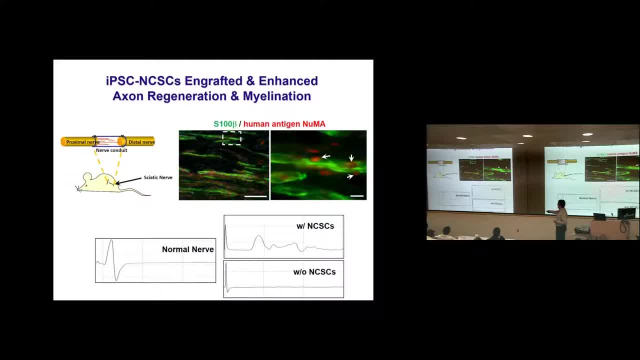 in the middle of the section you can see actually the aligned axon regeneration, especially all the all these green tunnels which are my melanated axons And human cells actually participate in this regeneration process and making all those melanation structure. 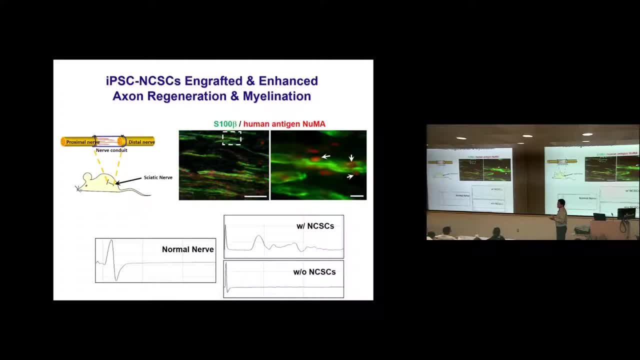 So if you do some electrophysiology at one month after surgery, you will see. actually, you know, with stem cells plus all the delivery vehicle, the conduit and matri-gel or hydrogel delivery vehicle, you will see a very significant electrophysiology outcome. 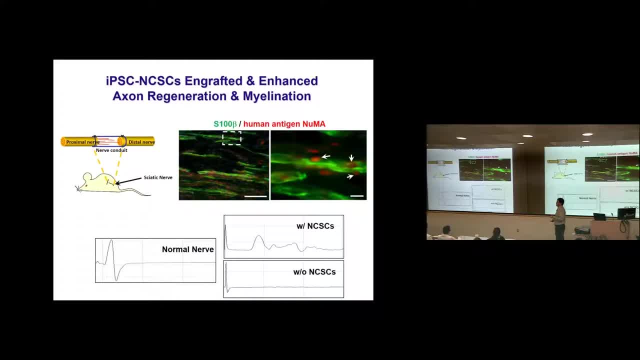 versus in the conduit, empty conduit without stem cells. you don't see that. So this study means you know we can generate a multipotent stem cells. In this particular case is a Schwann cell precursor cell. You can transplant these cells in the nerve regeneration model. and these transplanted cells can help peripheral nerve regeneration by producing more melanation, so which helps actually the axon elongation and helps the electrophysiology outcome. So in this rat model or immune, deficient animal model, rat or mouse models, you can look at human stem cell function. 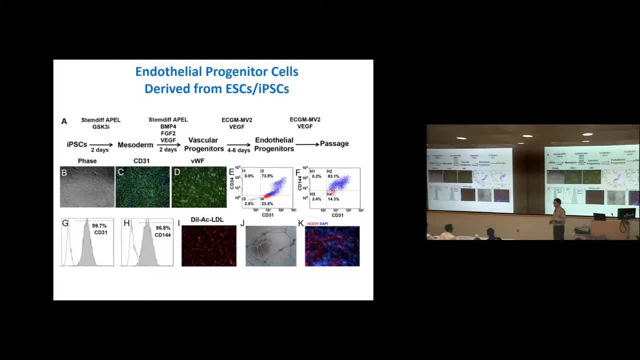 So all the immune system is blocked and the human cells will behave in the way that they would behave ideally in the human transplantation cases. So this is another example. very briefly, we can also differentiate iPS cells, or embryonic stem cells, into endothelial progenitor cells. 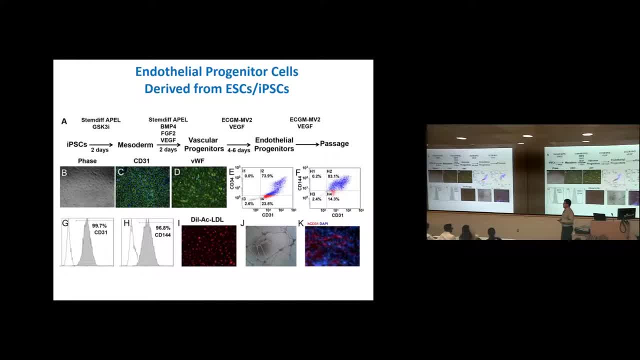 This is a collaborative project with Dr Jane Novotov's group, Dr Ping Zhou, an assistant professor in the stem cell program. So we're deriving human-specific iPS cells, derived endothelial progenitor cells. So you go through very similar to the other study. 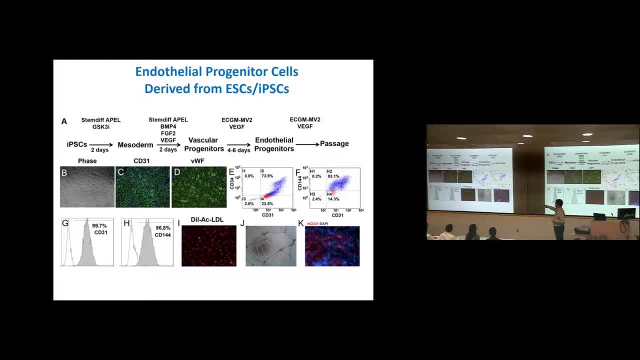 we establish a protocol. going through the differentiation process You get the endothelial progenitor cell at the last. So all those cells, they show very pure endothelial markers like CD31, VWF And also they actually can make tubes like tube formation. 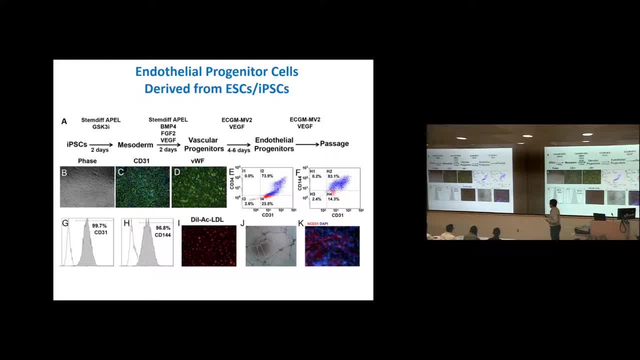 and they can uptake LDL. And in the animal model transplantation model we actually found that human CD31 is a human endothelial cell marker. They form some blood vessel structure in the. this was done in an NSG immune, deficient mouse model. 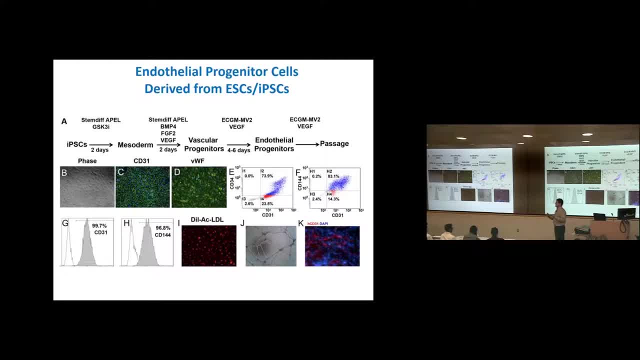 subcutaneous injection of a hydrogel loaded with iPS cell EPCs. So these cells are able to make endothelial cell structure in vivo and make blood vessels. So this is not a disease model, but this shows the potential of those iPS cell-derived cells. 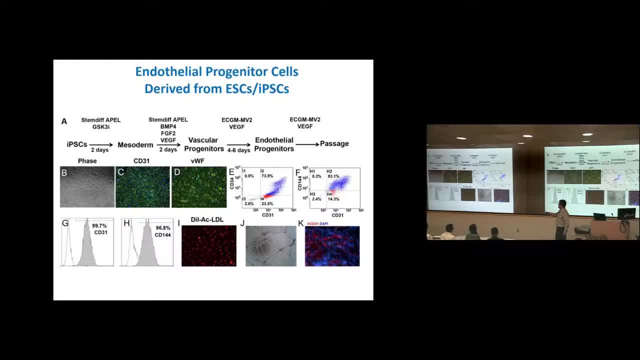 So if you think about from the top to the end, you actually get some human-specific iPS, cell-derived endothelial cells. You can get iPS cells from many different sources, as I mentioned earlier, skin biopsy, for example. You can get plus EPCs from skin biopsy. basically. 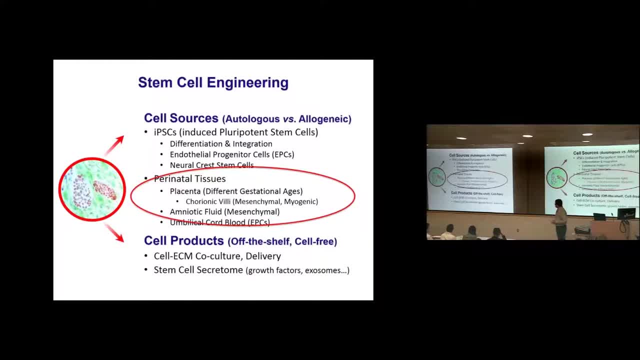 And you can use EPCs for many different applications. So the second portion of a cell source is a perinatal tissue that we have been working on for the past over five years. So placenta, especially, is usually discarded when the baby is given birth. 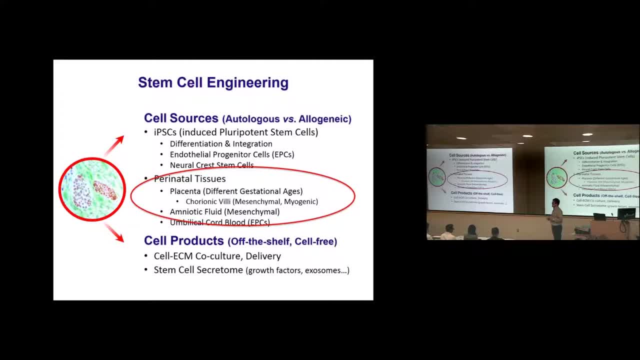 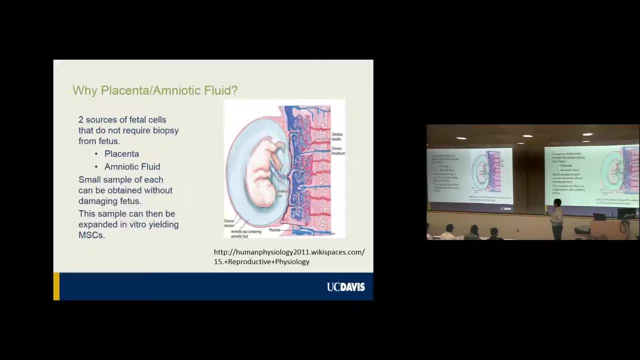 But placenta tissue is also available from different gestation ages- by biopsy actually- And amniotic fluid is another source If you think about how the baby is located in the mom's womb. so there are two sources of fetal cells that you can get without disturbing the fetus. 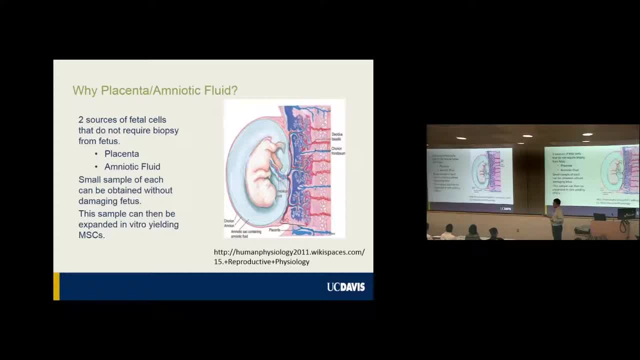 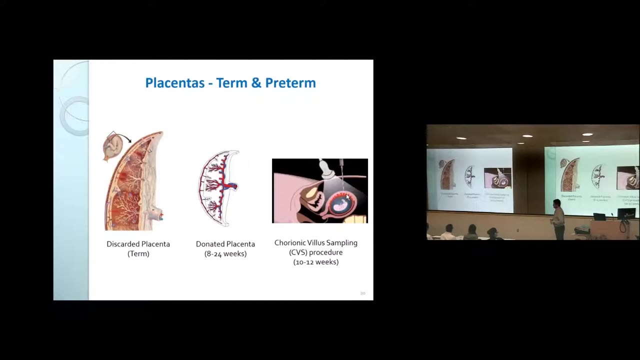 So one is a placenta biopsy, The other one is amniotic fluid amniocentesis. So both these samples can be obtained at birth, but you can also get those tissue samples from early gestation. So for placenta especially, we're very interested in looking at this step. 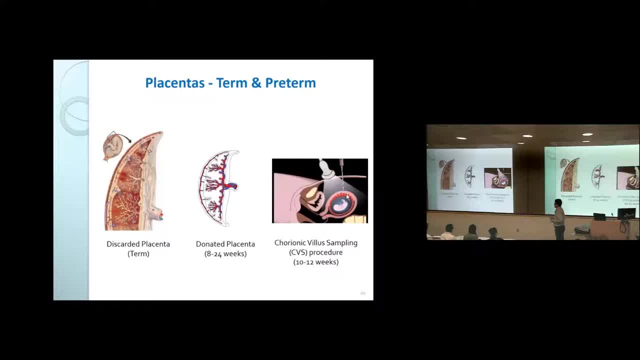 for stem cell, looking at placentas as a source for stem cells. So, as I said, discarded term placenta or donated placenta, mid-gestation, early mid-gestation or coronary villus sampling, which CVS, is a first trimester placenta biopsy technique. 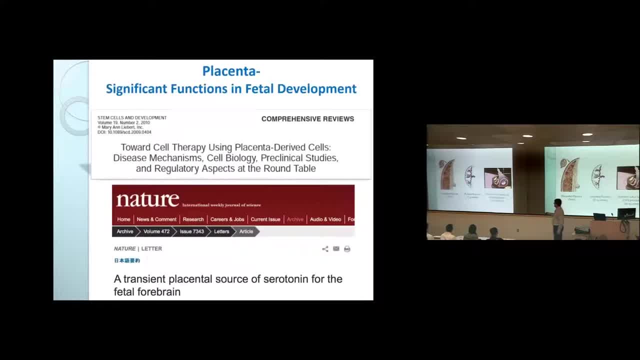 that is usually used for fetal diagnosis. So we can actually we know that placenta is very important for development in placenta during the whole gestation. So, for example, if you look at placenta in the gestation stage, they are very important in making many different things for development. 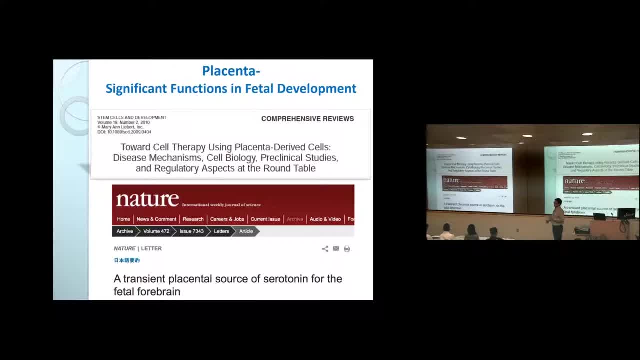 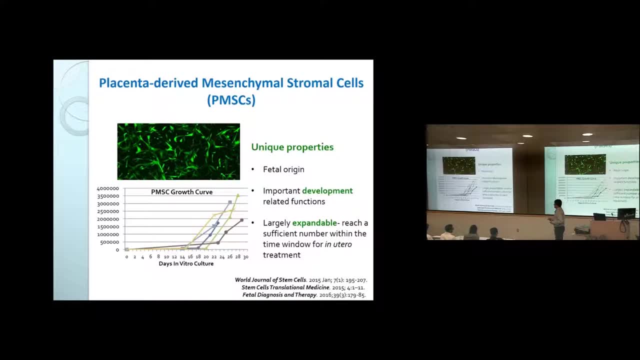 So, for example, there's a paper published in 2012 about this serotonin secretion from placenta. So if you block placenta serotonin source, actually the fetal forebrain development will be blocked. So in our lab we have established a protocol to isolate mesenchymal stroma cells. mesenchymal stroma cells. 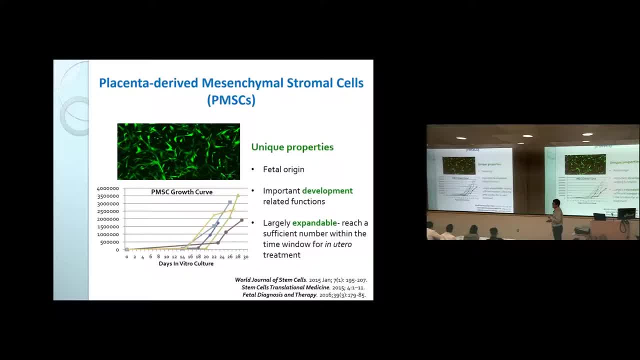 from different gestational stage placentas. This is a CVS age placenta which is about 9 to or 8 to 11 week gestation, Although the CVS tissue is very, very tiny, it's only like 30 to 100 milligram tissue. 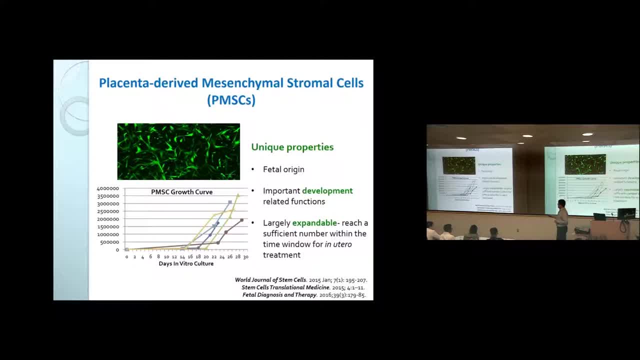 but we have established a protocol to expand cells into a like many, many millions of cells within like three weeks. So these cells are unique. they have many unique properties. Number one is that these cells are fetal origin, so which means you can use these cells autologous. 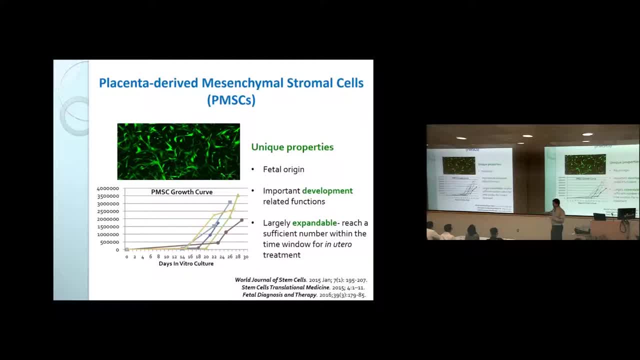 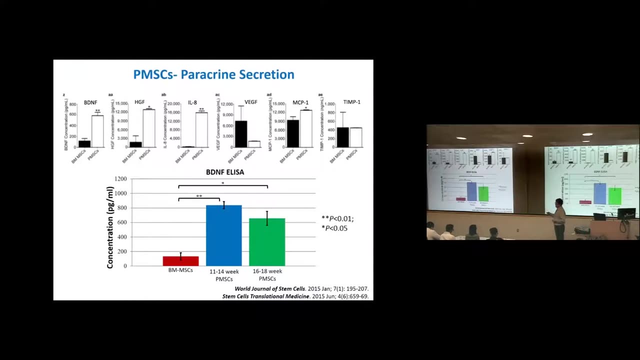 as an autologous cell source for fetal treatment or postnatal treatment. So it's a very unique autologous cell source And they're fetal, meaning they are very early, early in gestation, in development as well. They are very expandable and they are secreting a lot of very important factors. 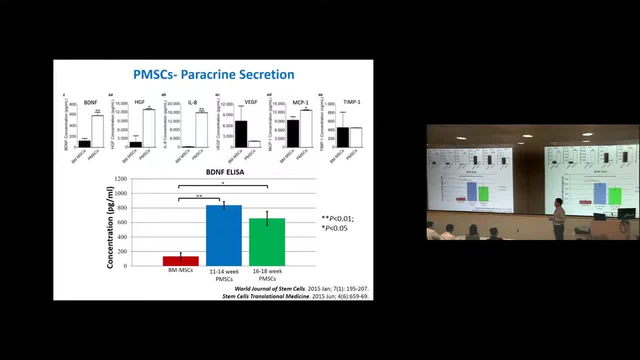 growth factors, cytokines- very important for development and for healing. As we all know, fetal environment is very pro-healing- and all those placenta-derived early gestational stem cells. they are actually very important. they're very secreting many very important factors. 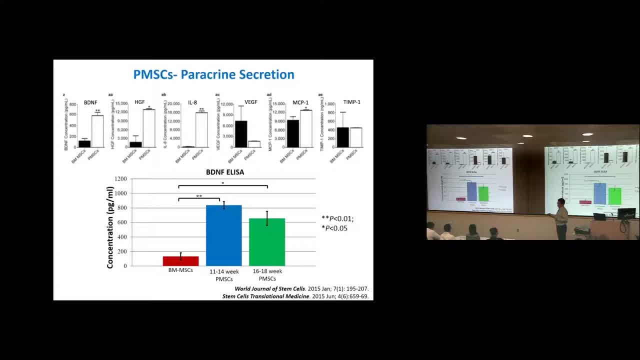 For example, we're looking at BDNF- brain-derived neurotrophic factor- is a very powerful neurotrophin, very important for brain development and spinal cord development in development And also neural survival. So one thing that we discovered that many, many in vitro work has like studies have been done in the lab. 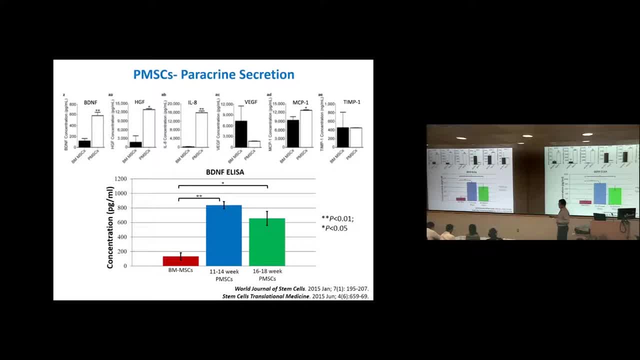 one thing that I want to mention today is the BDNF secretion level. Actually, if you look at adult bone marrow, they're all MSCs, so you can generate MSCs from different sources like adult bone marrow. that's very, very often done. 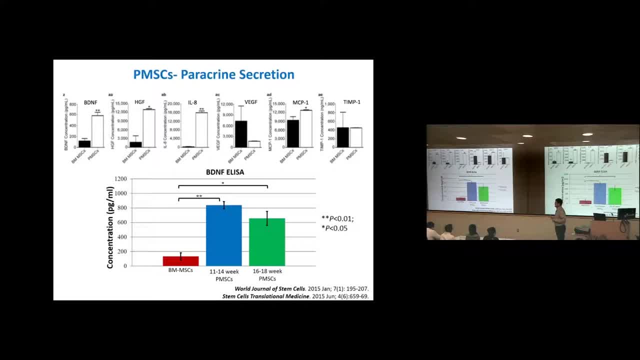 and our stem cell program here has a fantastic bone marrow MSC product, a different series of products for different diseases. But if you compare placenta MSCs with the adult bone marrow MSCs, you see much higher level of BDNF secretion in the placenta MSCs than adult MSCs. 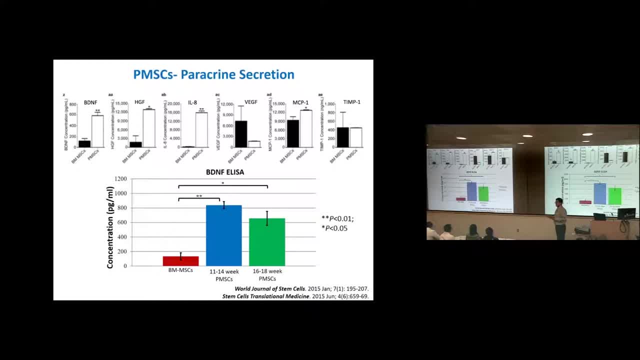 So one thing that Dr Nota, our stem cell director, stem cell program director here at UC Davis. one project they're doing is to make adult bone marrow MSCs to secrete high-level BDNF for Huntington disease. What they're doing is to transduce bone marrow MSCs with lentiviral vector to overexpress BDNF. 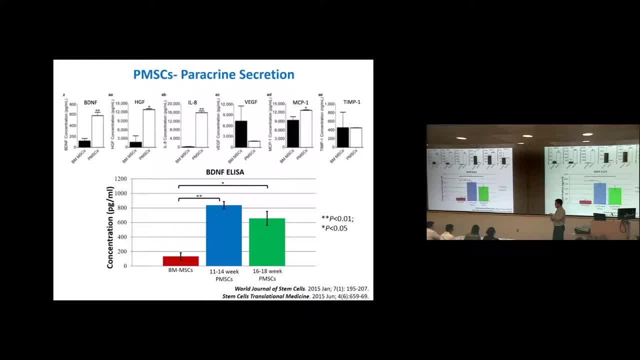 So actually in our case, the placenta MSCs are naturally secreting high-level BDNF, so you don't need to do any gene delivery or virus manipulation for those cells. Potentially, these cells are very useful for many BDNF-related applications. 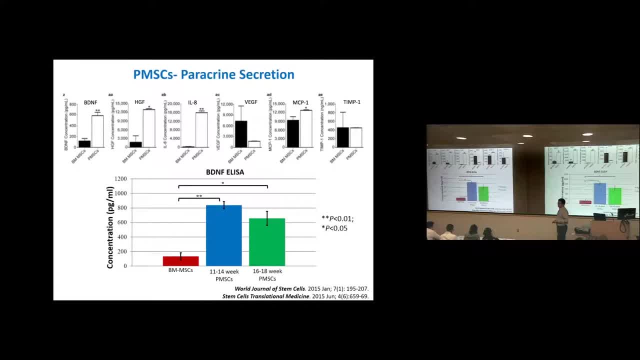 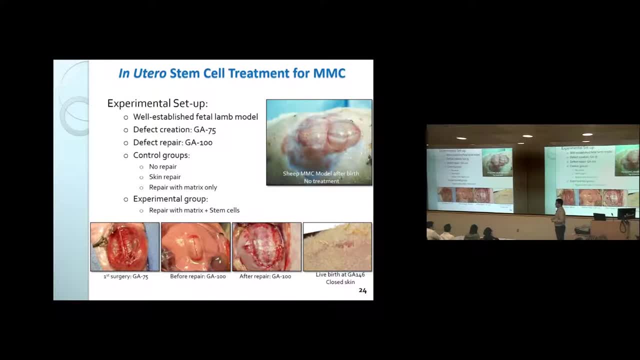 brain, spinal cord, many other neuron survival-related applications, But this is just one side of it. Many other factors are able are secreted by placenta, MSCs- actually that you can like. VIGF is pretty high level as well, and HGF is also very highly expressed. 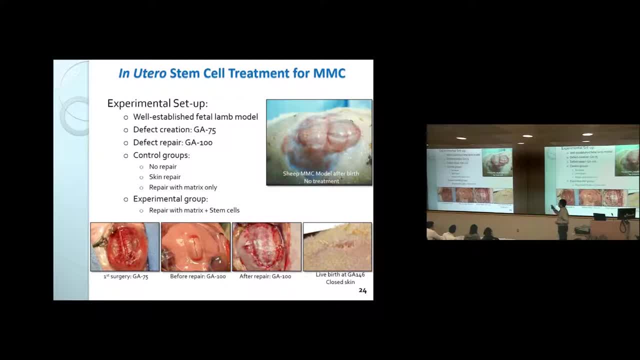 in placenta MSCs. So we have transplanted these placenta MSCs in the fetal sheep model of spina bifida. that this is a major collaborative project between Dr Farmer and myself and the whole lab, surgical bioengineering lab, supported by CIRM and Schreiner grant. 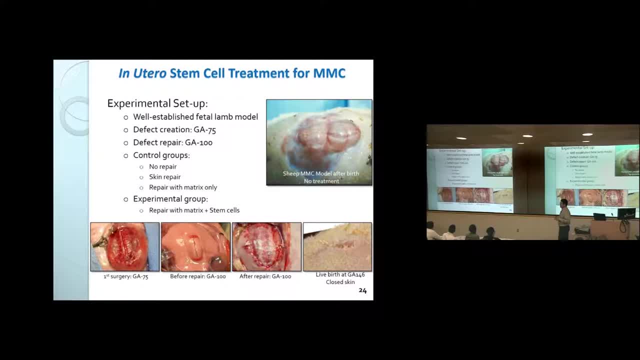 So basically we're looking at how we can supplement the fetal surgery. As you all know, fetal surgery can actually treat spina bifida- spina bifida very well before the baby is born. but can we do that better? Can we supplement the fetal surgery with stem cell products and make these patient outcome better? 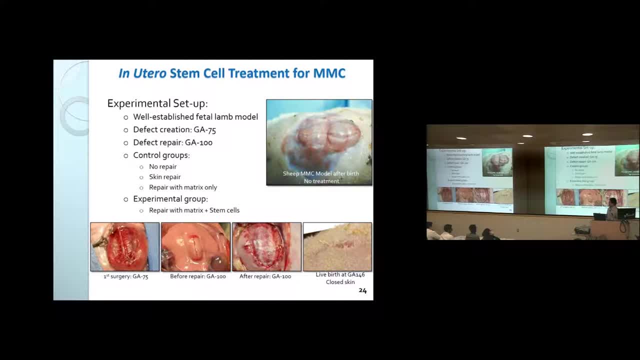 So we actually we have this. we just transplant these cells into this animal model at the secondary surgery, which is, you know. you know that this model is the first surgery of GA-75, and then the second surgery is the GA-100, and then, 45 days later, the baby lamb will. 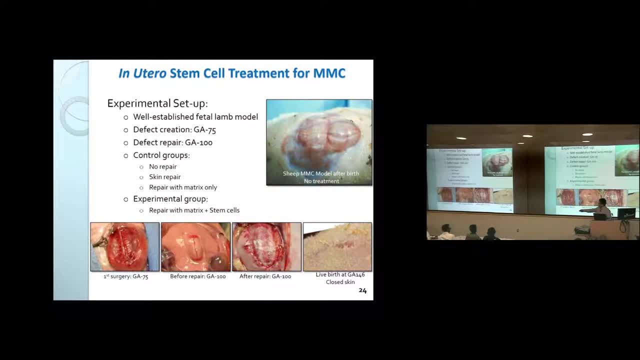 spina bifida, baby lamb will be born. So when we transplant cells here at the second surgery, when we do fetal surgery, we add a component which is stem cell product. So in this particular case we have placenta MSCs co-cultured with an ECM matrix. 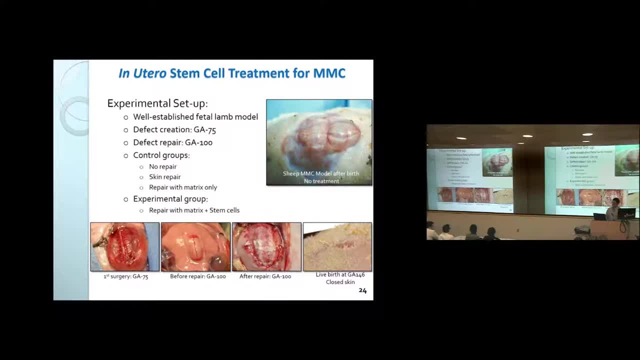 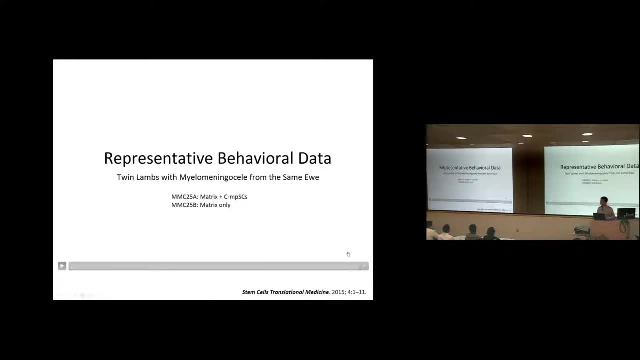 a scaffold sheet that we can patch the defect with. And so here, actually, I'm going to show you a very short video that I believe most of you have seen that before. It highlights the importance of the stem cell function in the stem cell. 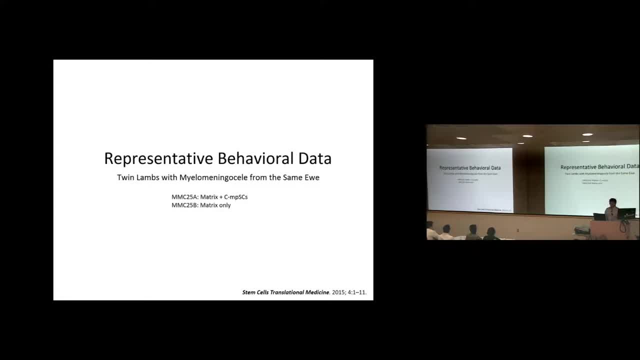 So the stem cell function is a very important part of the fetal regeneration environment When you have so. we have two twins. one was treated with stem cells plus matrix. the other one was treated with matrix only without stem cells. As you can see right at birth, this is the beauty of the lamb model, right at birth. 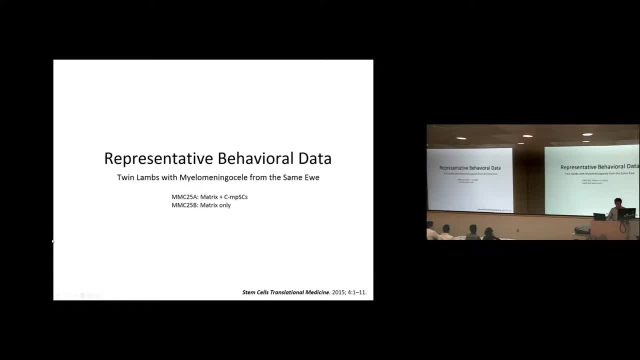 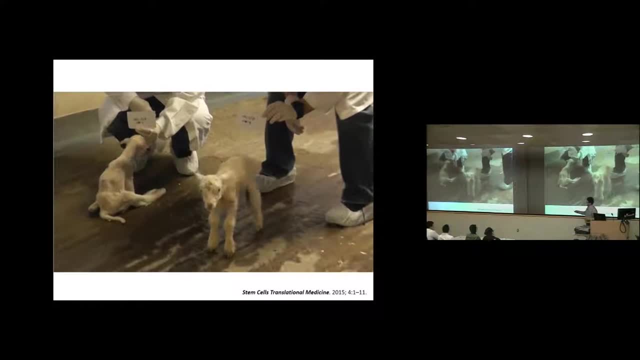 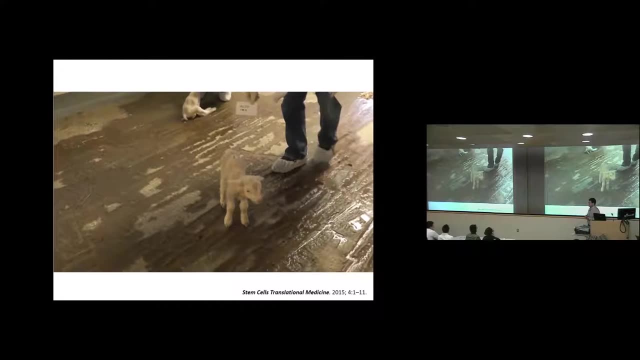 the lamb would be able to stand up and walk, if they are able to. So in the spina bifida lamb they develop very typical paralysis and this is the gold standard animal model for spina bifida research. But this lamb was treated with the stem cells plus matrix. 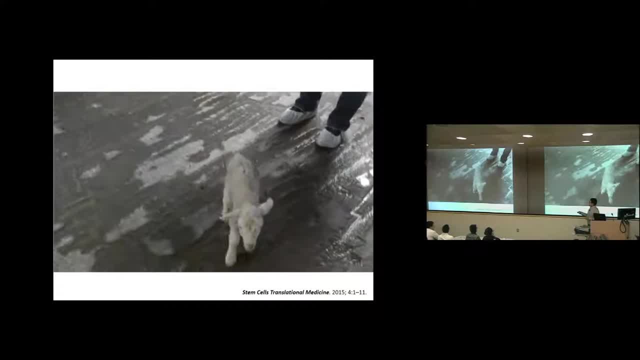 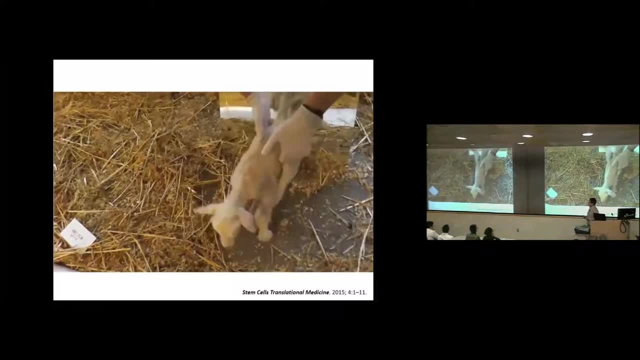 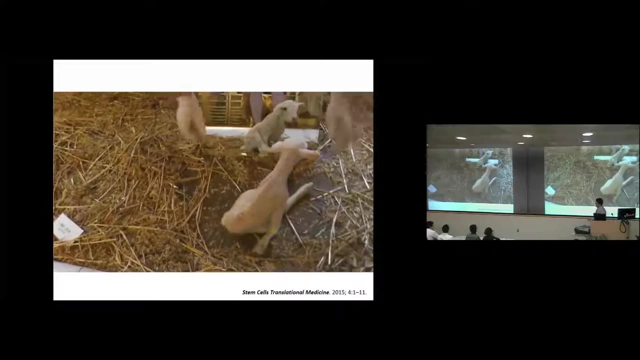 So the other one was treated with matrix only. So we have seen, you know, this lamb actually was able to stand up and walk just normally And the other one was developing very typical paralysis associated with the spina bifida, And this treated 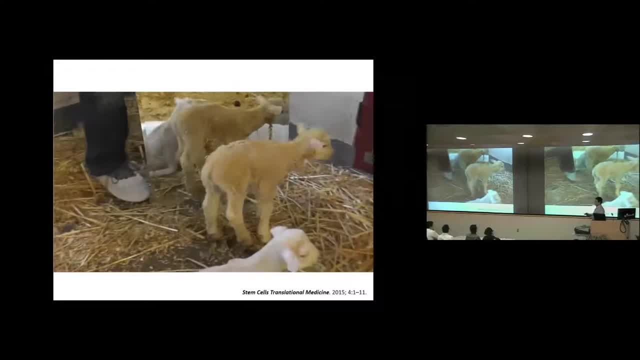 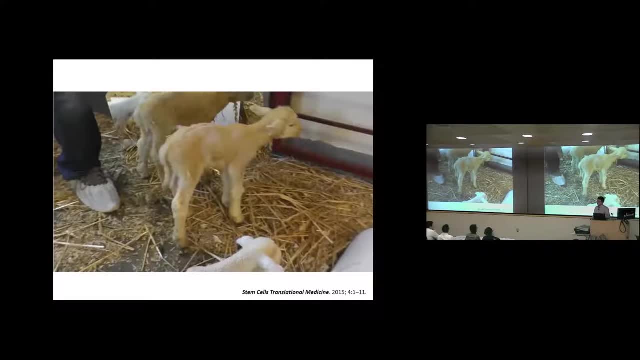 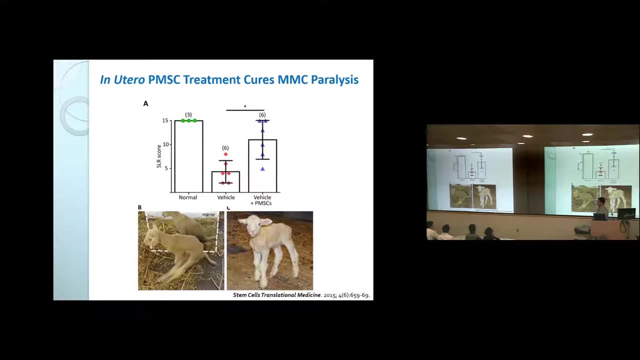 stem cell treated animal actually was able to stand up and walk. in coordination, very nice coordination, all the limbs and tail, movement and nerves, everything is just normal. So what? we and we've done this. many, many sheep actually- now I have more numbers than this now. 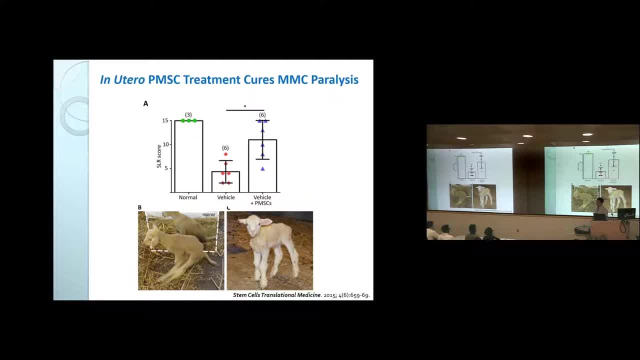 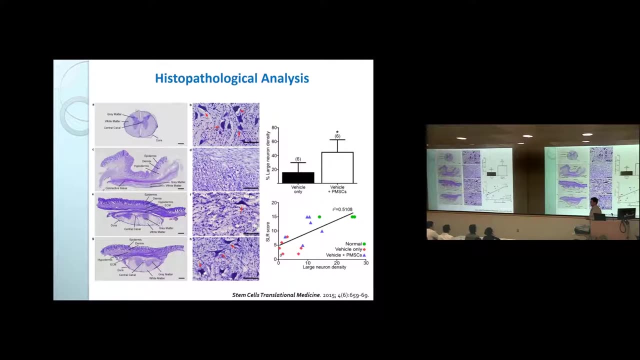 But generally speaking, we found that this recovery or this stem cell mediated regeneration effect actually is a very reproducible and consistent. So we hope that these cells are able to, you know, develop, we're able to develop these cells as a product in the future. 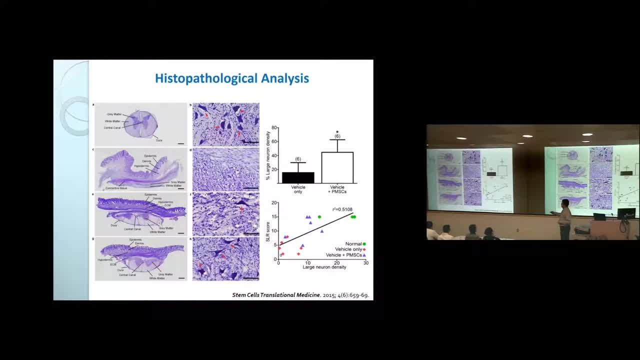 So we did some histology. If you look at, this is a normal spinal cord. If you look at the butterfly structure with the gray matter where the all the neurons are located that you have, you can see a lot of very normal phenotype of large neurons there. 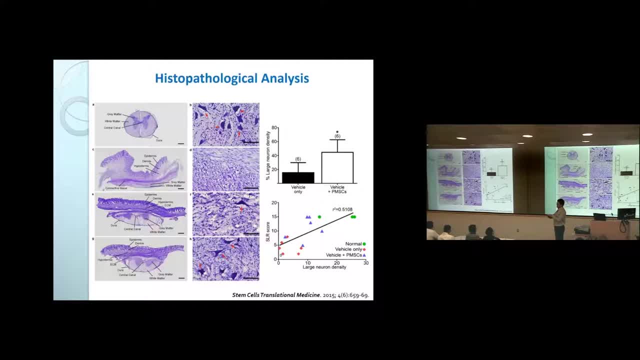 And this is a skin repair, which is a mom's trial skin repair, fetal skin repair. You see some preservation of the core tissue but very, very few neurons that can survive in the whole process, actually, at least in this animal. 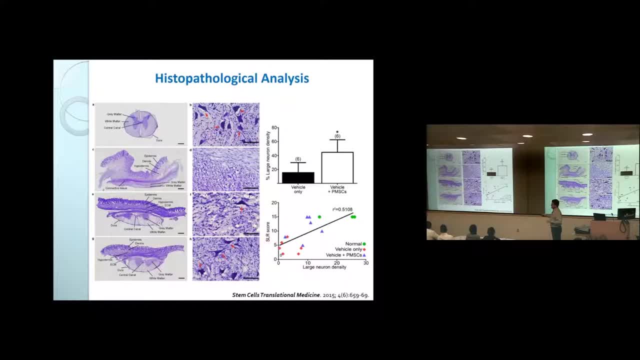 And so this is one. this one is the ECM scaffold, only without stem cells. You see some neurons actually, which means the ECM scaffold is plus. fetal surgery actually is helping the recovery in the spinal bifida. But now that's good at this group. 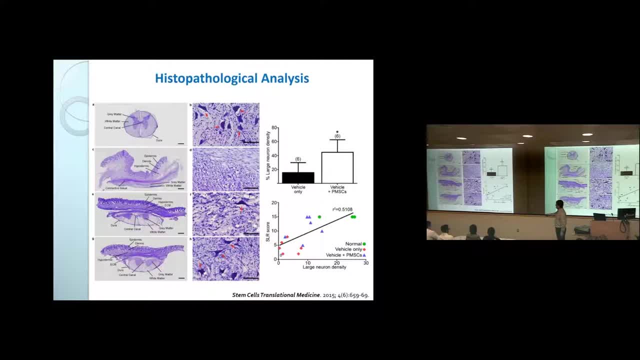 This is the ECM plus stem cells. In the gray matter you'll see large density of neuron- very high density of neurons- actually survive- And vehicle plus PMSCs. you see the large neuron density is much higher than the vehicle only And you see a very pretty linear correlation between the neuron density. 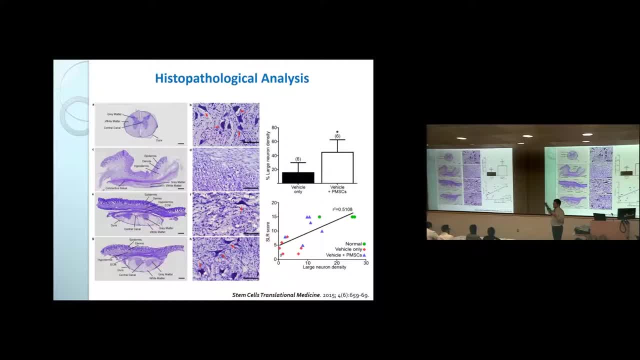 and how well the animal was able to walk, which means the better neural preservation, the better the animal will be able to walk. It's very, very important. It shows the importance of the stem cell function in this particular case: neural protection or neural preservation. 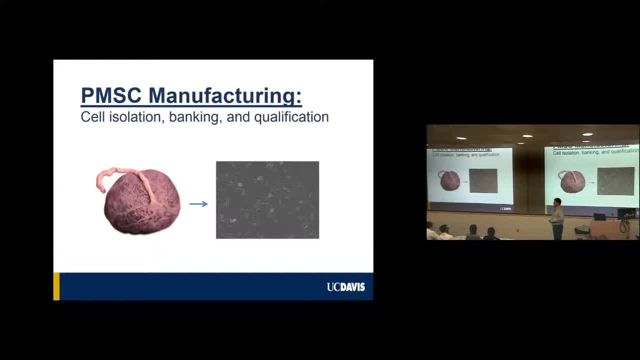 So now we are- actually we're still doing a lot of sheep. now We are basically trying to figure out the dosing, We're trying to figure out how to deliver the cells better, what the protocol or product is, the better, And also we're developing protocol to make a cell product. 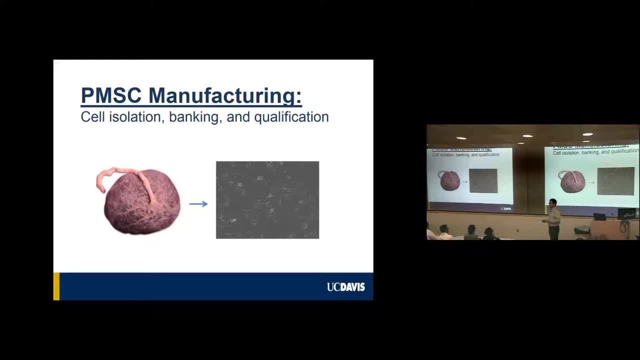 So we are using all these GMP, good manufacturing practice, associated procedures, reagents. We're making a cell bank, So we're making a cell bank. So we're making a cell bank. Basically, that can potentially be used for off the shelf. 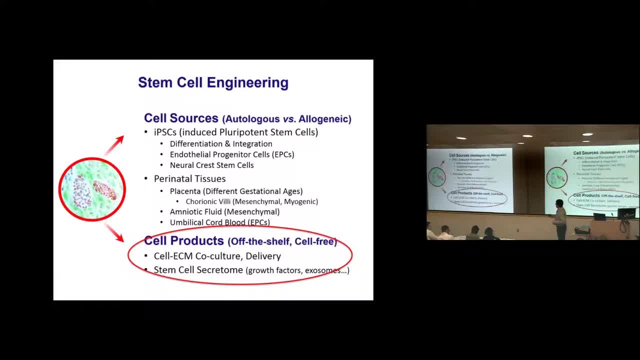 for different patients. So that actually is going on very actively in the lab right now. We're developing many, many cell lines and many, many vials. So hopefully at the end of our current CERN project- it's a preclinical development award. 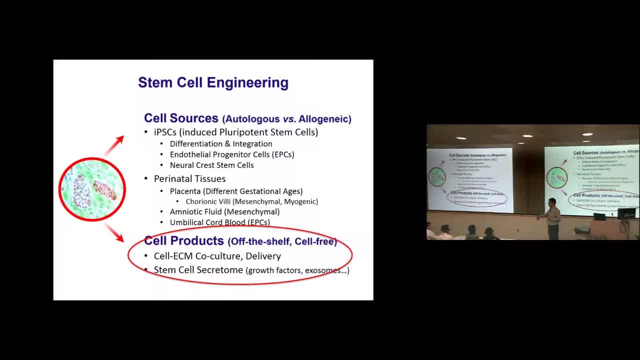 So at the end of this project, or close to the end, we're going to apply for another grant. Hopefully we can get a translational clinical research grant so that the stem cell product can be applied into some clinical applications. So, as I said earlier, we're also making a lot of cell products. 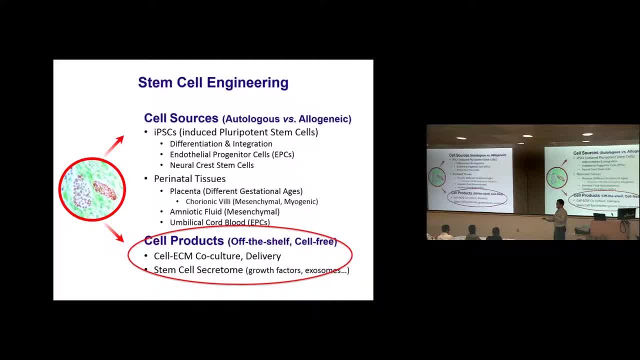 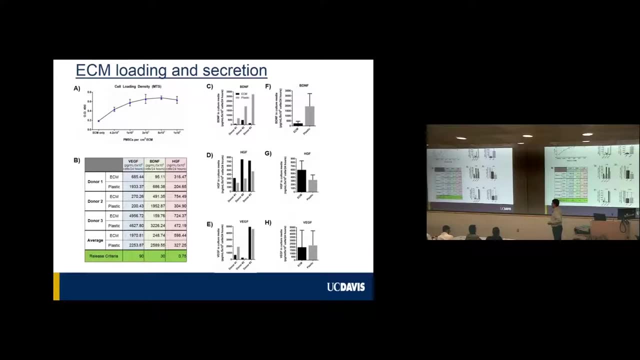 like a cell ECM- co-cultured cell ECM- as a patch material that can potentially be used for many, many defect treatment. We're also looking at the stem cell secretome, stem cell secretion, growth factors or other things like exosomes. 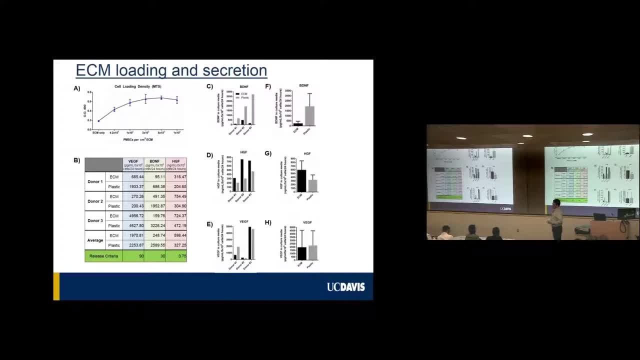 So we're looking at the ECM loading and secretion. so how the extracellular matrix scaffold, the clinical grade ECM product, how the stem cell can be loaded on the ECM, how they behave in vitro and in vivo. So one very important thing that I think to my opinion. 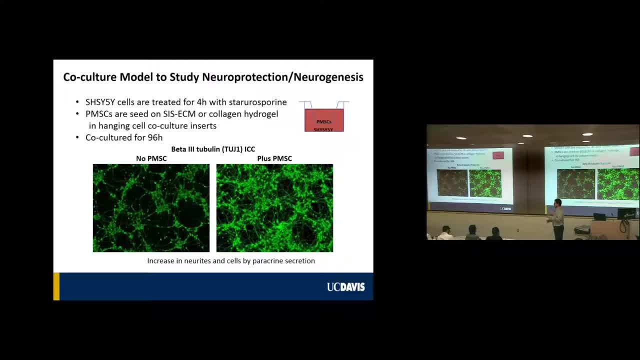 is the some in vitro model to test how your cells are. So, instead of using a very expensive animal model like the sheep model, if you have a platform that you can use in the lab to test the cells, which cell line is better, so that would be fantastic. 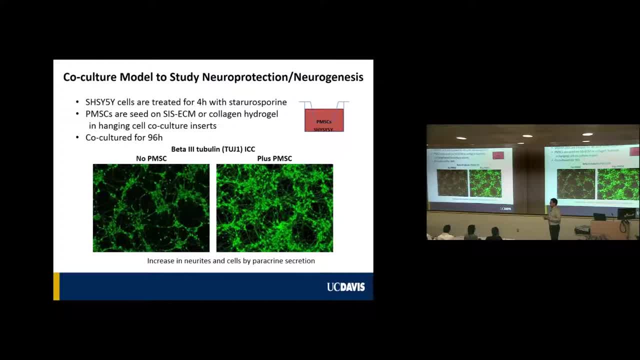 I mean, everybody is trying to establish some vitro cell screening model. So in our lab we establish a neural protection model. Neural protection is considered one of the major mechanisms for the spina bifida fetal surgery repair. So as we can see in this model, basically we 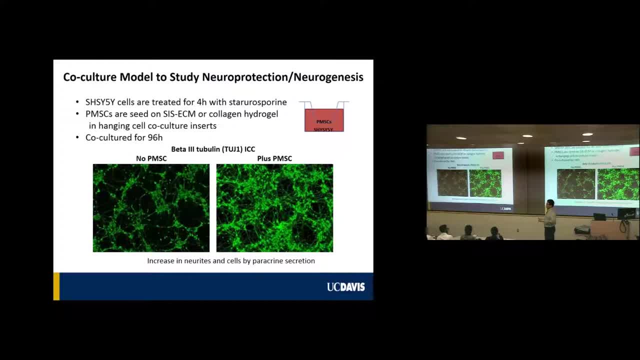 develop a neuron, a blood soma cell line, which is a human neuron cell line. You culture these neurons here and then you damage these cells, And then you apply different cell lines and see which cell line can protect the damaged neurons better. So we, for example, we see very consistent protection. 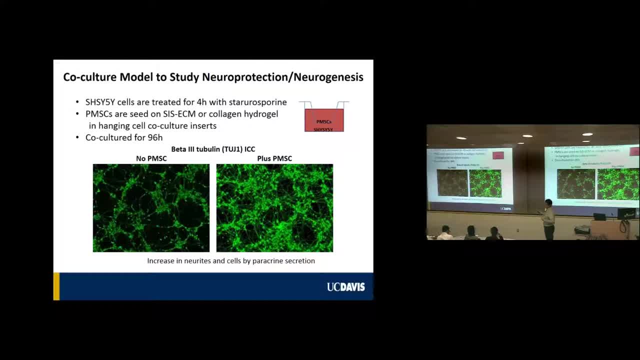 between cell lines, with or without PMSCs. Generally speaking, with PMSCs- placenta, MSCs- more neurons will survive. They've developed better neural network. But between different cell lines, different cell lines from different donors, different cell lines. 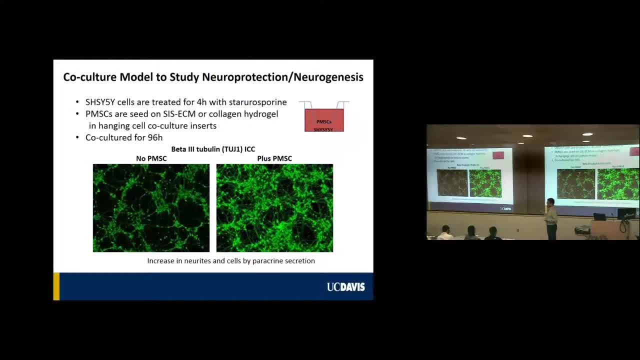 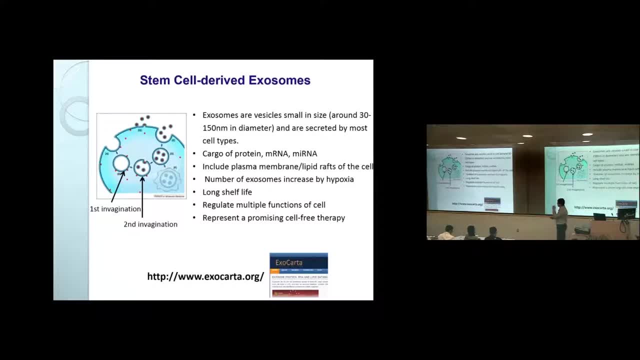 from different gestational ages, the protection effect is different. So we're using this as a in vitro model between screen cell lines, basically. So another thing that we're doing very actively in the lab is the stem cell-derived exosomes. As you may know, exosomes are some nanoparticles. 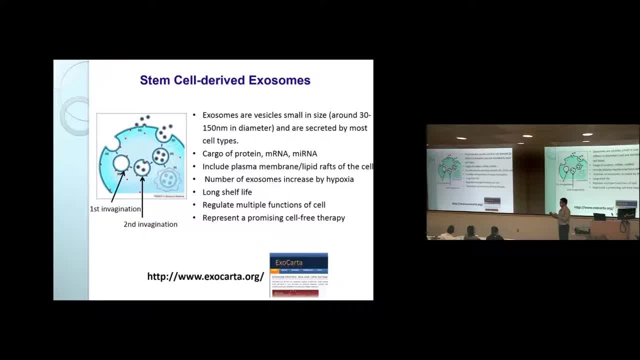 secreted by cells and that can mediate cell-cell interaction. That's how the cells that are apart, very far away from each other, how they sense the other cell communication or the other cell function or need or those kind of things. It's like a cell phone or a smartphone. 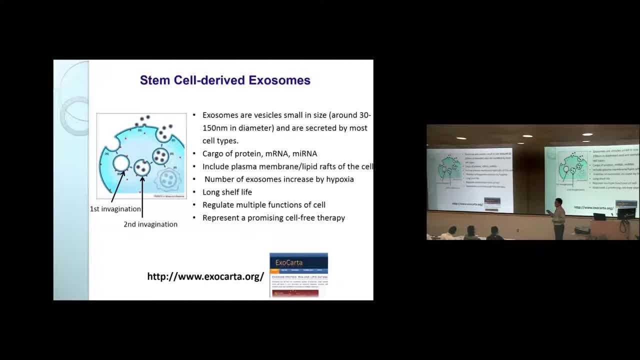 That's what Dr Jan Notas' group has been calling exosomes, Like you call the other cell far away from you, without giving direct touch. but you can give this information by exosomes. So exosomes are secreted naturally, normally by cells. 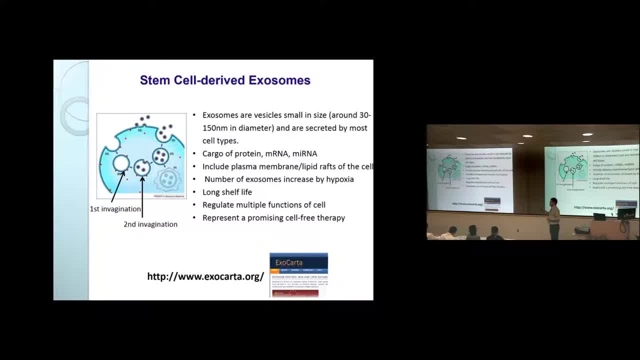 And these exosomes can be taken out by other cells. So different cells in different environment, different cells may pick up different exosomes, But in our particular case we want to develop steps where we can develop stem cell exosomes. The main reason is based on our sheep study. 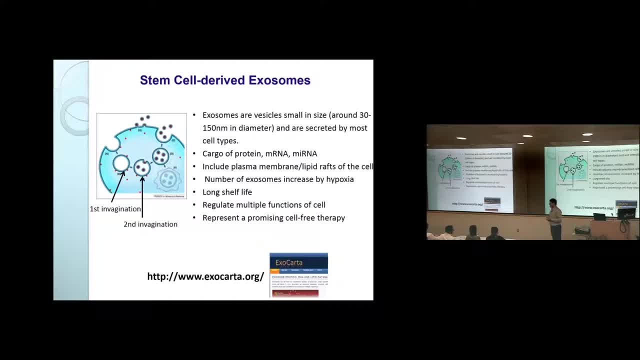 that I didn't mention earlier. So from histology we noticed that there are no human cell engraftment at 45 days after transplantation. But the lambs were able to walk. So what's going on between these 45 days? 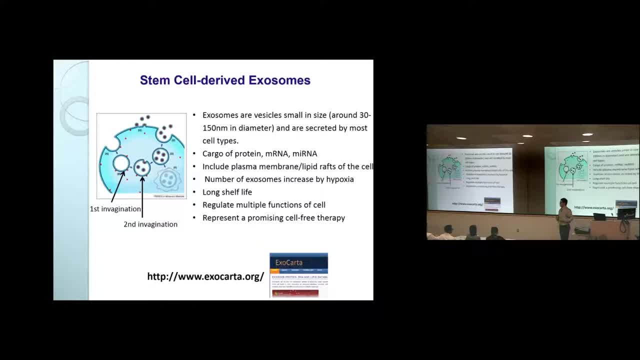 We have done multiple time points lamb histology, But basically we concluded that the transplanted human cells they don't stick around long, They don't stay there for long. My guess I don't have a very firm conclusion on how many days exactly they stay in the environment. 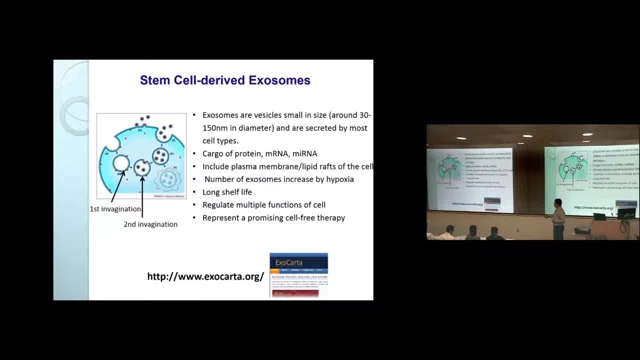 My guess is about two weeks, two to four weeks, But they disappear over time. But they've left a lot of very important factors or stuff where they stayed Exosome. that, we believe, is one of the major products that the cells secreted. 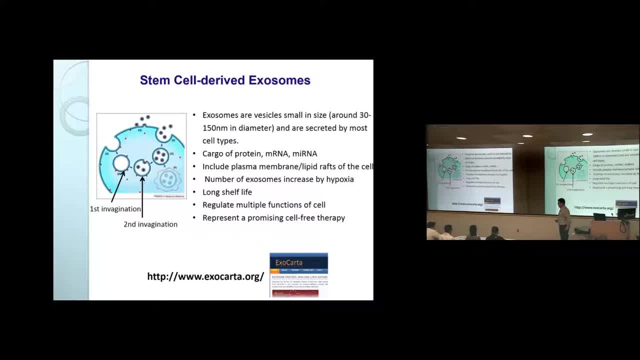 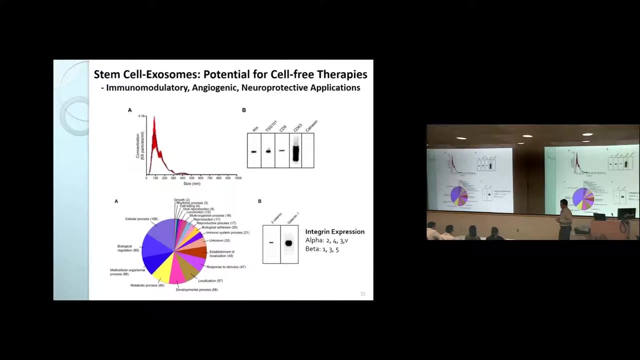 And then they're gone. They don't leave, But they left those important components there, All those exosomes secreted by the transplanted cell. they can be taken, eaten by other surrounding cells, for example neurons. So we have shown this actually in vitro in the lab. 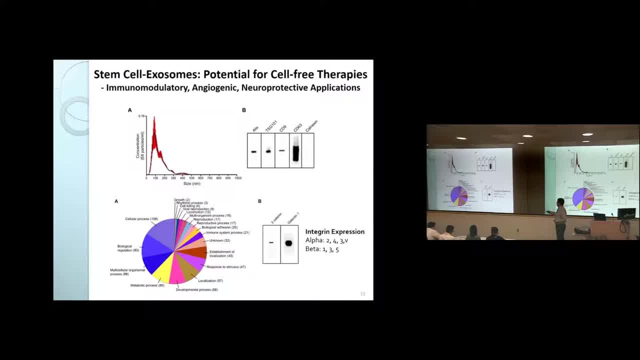 We have a large scale culture: PMSC, placenta, MSC culture. We established a protocol to isolate exosomes from culture. They are nanoparticles. You can use many different ways to isolate these stem cell exosomes. You see very, very many, many proteins actually. 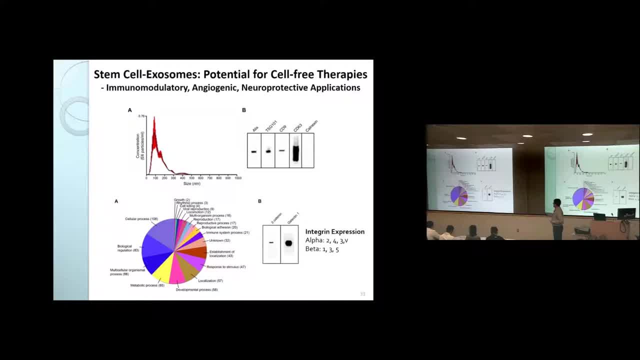 are contained in exosomes. You see many specific, some other very important proteins, for example Gallatin-1.. So I can't go into any details for here, But there are many, many important studies about Gallatin-1 in stem cell transplantation applications. 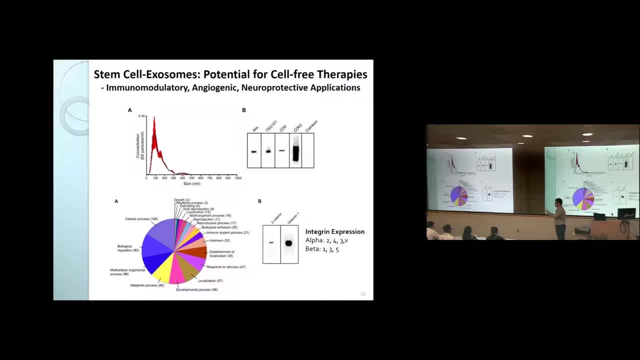 So these exosomes, stem cell exosomes. they are actually expressing high level Gallatin-1.. And there are many other integrin, very important cell surface proteins are expressed on the exosome surface, which means that's how the exosomes stem cell derived. 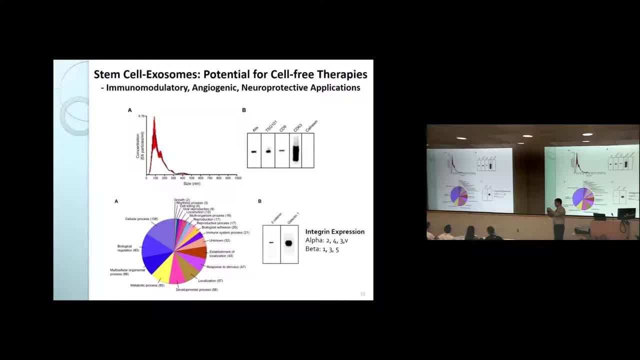 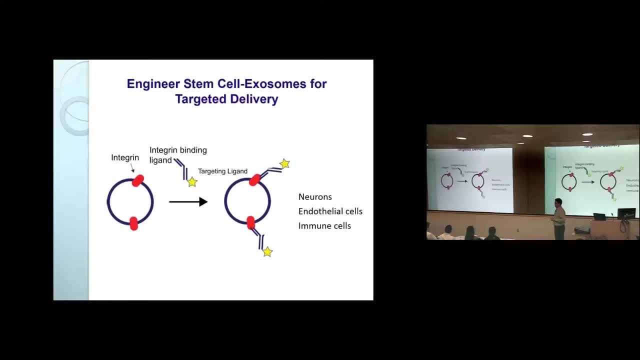 exosomes, particularly here how the exosomes are taken or eaten by other cells, by cell-cell binding mechanism basically. So we have one project very actively going in the lab is to so you can generate a lot of stem cell exosomes. 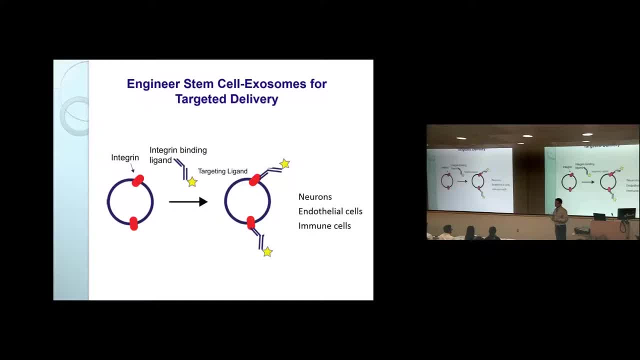 You can direct use these stem cell exosomes for many diseases because they are nanoparticles, They can. you can inject IV, You can localize, You can actually put the put those stem cell exosomes anywhere that you want, because there's no live cells related. 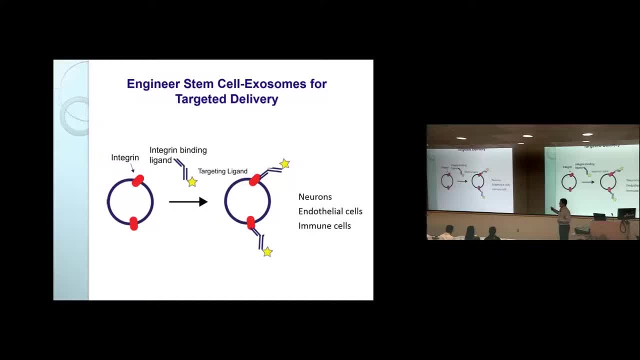 to this application to this end. So there are many other research, like projects going on about stem cell exosomes for different disease treatment that we just don't have the manpower in the lab to do that now. But what we want to do is to how you know. 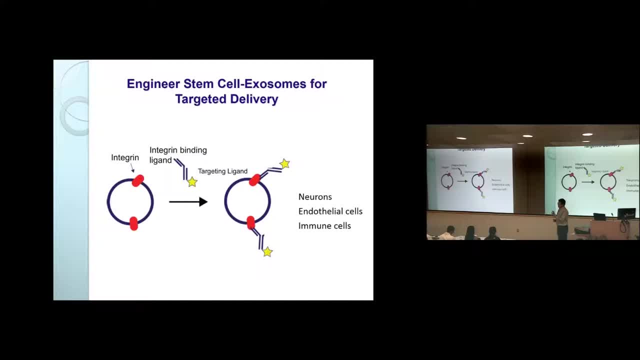 to engineer these stem cell exosomes and trying to make these stem cell exosomes more specific. For example, based on the surface marker expression, integrating expression, you can engineer and add some ligand to the exosome surface, make them different so that they can be eaten. 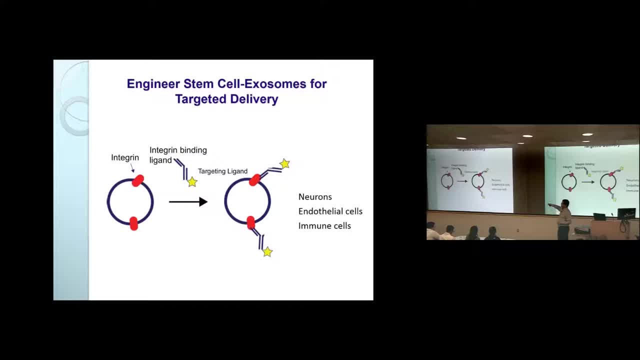 by certain cell types. more specifically, If the ligand is specifically binding to endothelial cells or neurons, so these stem cell exosomes will be eaten by neurons or stem cells or apoptotic cells or other cells, just based on your need or your design. 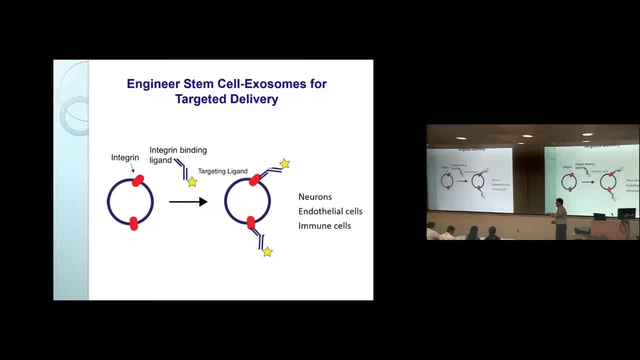 So they can be more directly eaten by certain cell types, So that they are. the effect will be hopefully higher the better, because the precious stem cell exosomes, so stem cells are making exosomes, but pretty low level compared with the cancer cells. 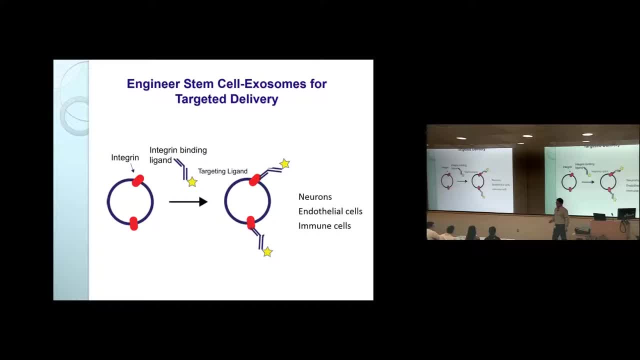 But how you can use these stem cell exosomes more effectively. that's a key thing. So we're developing this Basically. you can use these things for different applications. You can rescue neurons, you can rescue endothelial cells, you can target immune cells, you know. 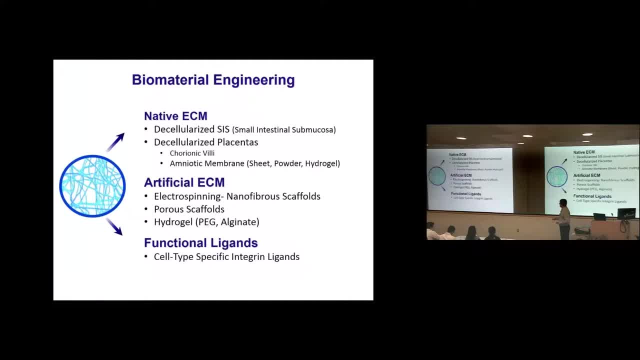 you can do many different things just based on your design. Very briefly about ECM, So extracellular matrix, as you know, you know the body is made of cells and extracellular matrix. So we're talking a lot about cells, but at the same time and on the same side. 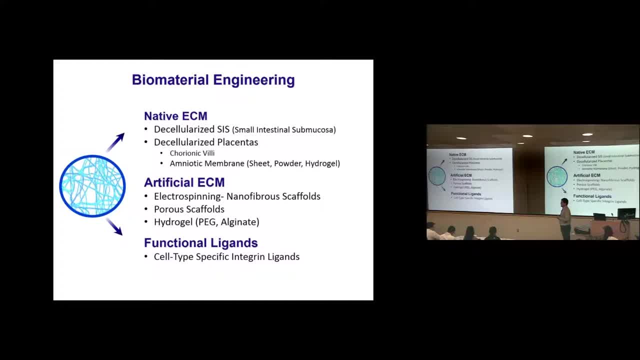 the other side is a cell extracellular matrix, so where the cells are living in. So you can get a lot of native ECM. native ECM by decellularization. You can also get some artificial ECM that you can make produce, You can make a lab to, or you know. 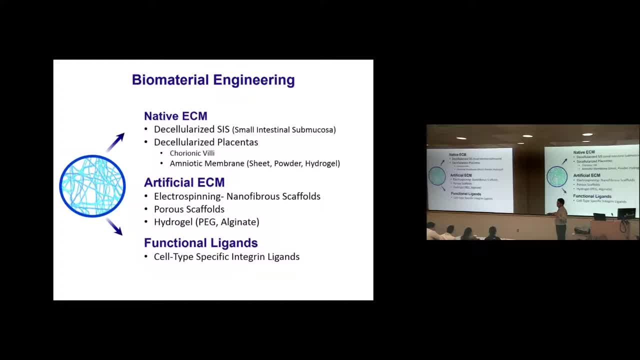 in a production site to make artificial ECM that mimics native ECM as much as you would like, And also the functional ligands that can be used to modify artificial ECM. So, artificial ECM, you can make them into different shapes, but they don't have any biological stuff. 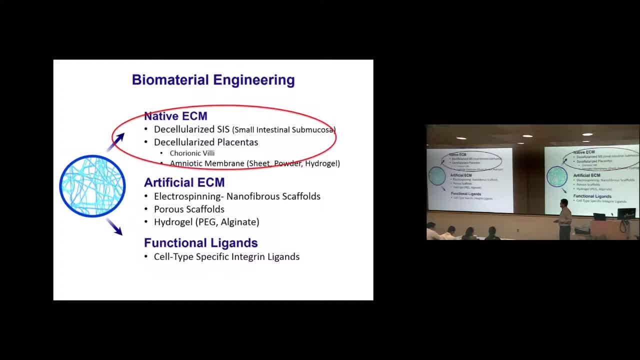 Then you can engineer the surface to make them more biologically active. So, ECM, as I mentioned, you know, earlier, in the sheep study, actually we're using a cook product that Doug Boyd actually is expert in: the decellularized SIS product from the pig. 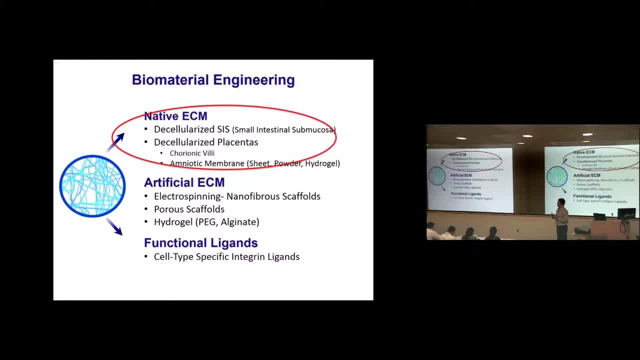 And so they're making the decellularized SIS into different formats- the sheet of material or many other formats like hydrogel or emulsified injectable format or some other things, And in our lab actually we are developing some human ECM. 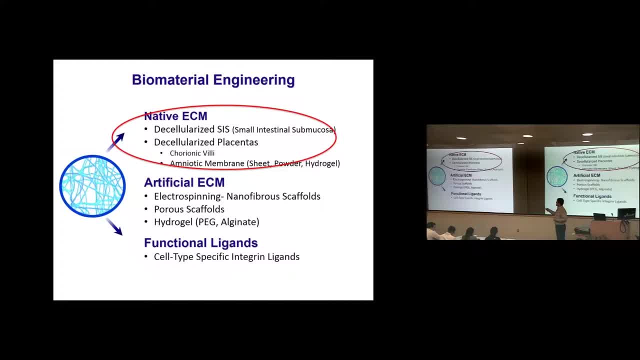 So, as you know, we're developing some human ECM. You know, all those ECM mainly are produced by pig tissue but they are from different species right from pigs. There are some rejection problem associated. May not be very significant, but ideally human ECM may be better. 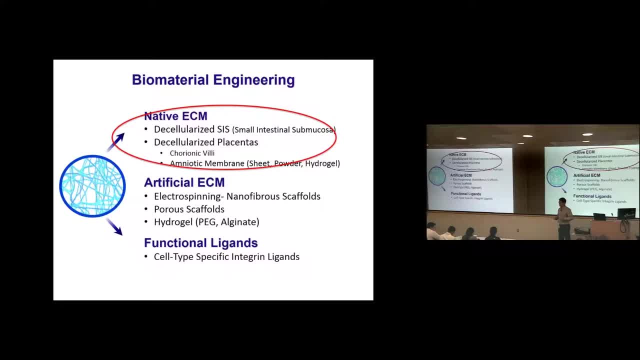 The reason we're looking at this is because we have lots of placentas in the lab and placentas are human or like tissue. They are discarded usually. So we developed a protocol to isolate cryogenic vet li, isolate. We have amniotic membranes and we decelerate these tissue. 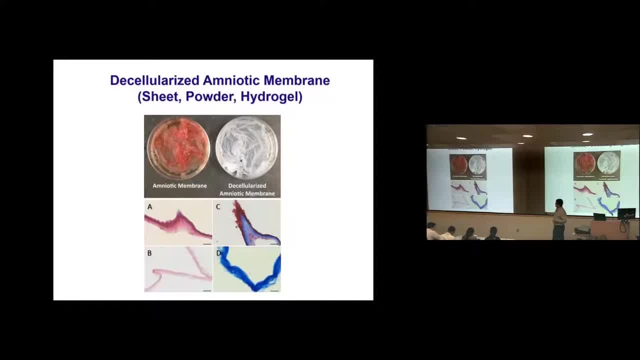 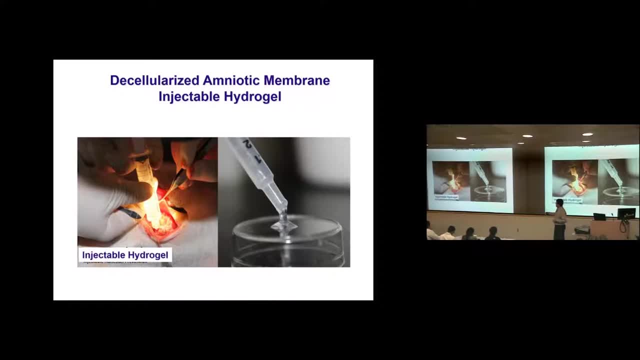 into ECM. So we have developed a protocol, As you can see very well, decellularized after decellularization, before decellularization, And we can also develop this into an injectable hydrogel. that actually one of our research residents, Ben Keller. 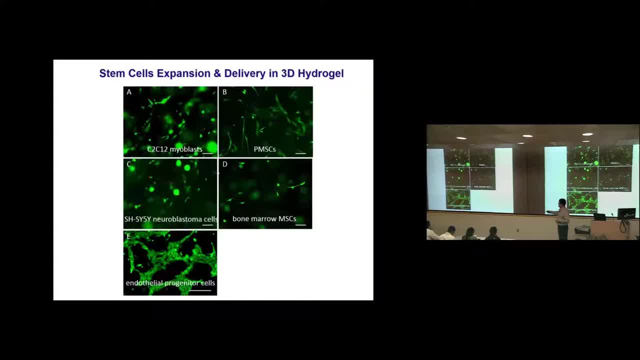 has been very actively involved in this project and another graduate student. So we can also use these injectable hydrogel- human ECM hydrogel- for human cell culture, expansion or delivery. So potentially we can use this as a product for many stem cell. 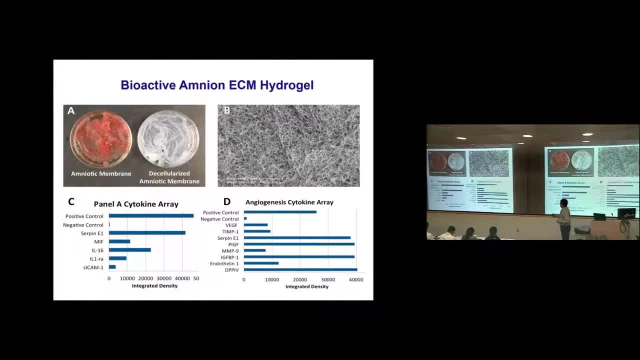 culture or expansion or delivery. And we also noticed that these human ECM hydrogel they are bi-active, They're not inert. They have lots of good stuff still in there. So the protocol is pretty mild. Most of the growth factors that we can still detect afterwards. 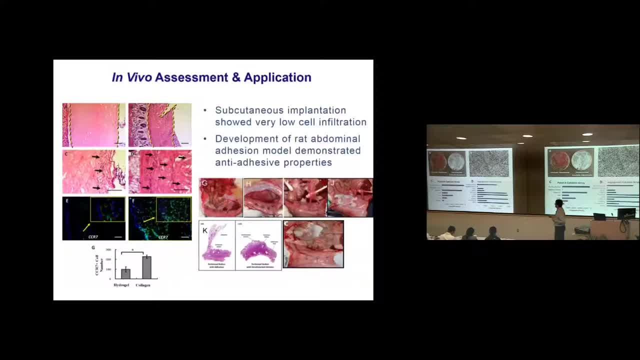 A lot of angiogenic cytokines are still present And we did some evivo initial testing that we're going to be doing more to confirm this. But in the initial study we found that actually compared with the bovine tendon collagen, as you can see. 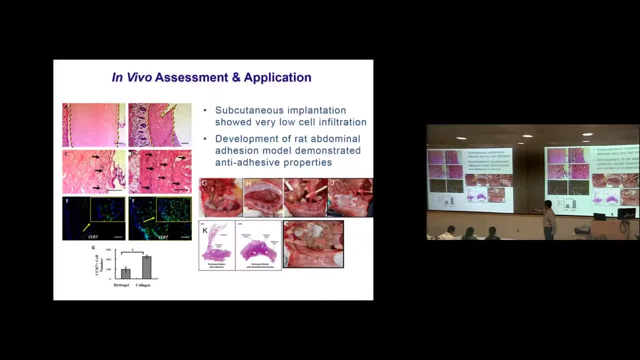 like two weeks after evivo transplantation. you see the tendon-derived collagen, bovine collagen. You see many more cell infiltration, many more cells infiltration. You see many more cells infiltrating into this collagen. hydrogel, This is a hydrogel, This is a hydrogel. 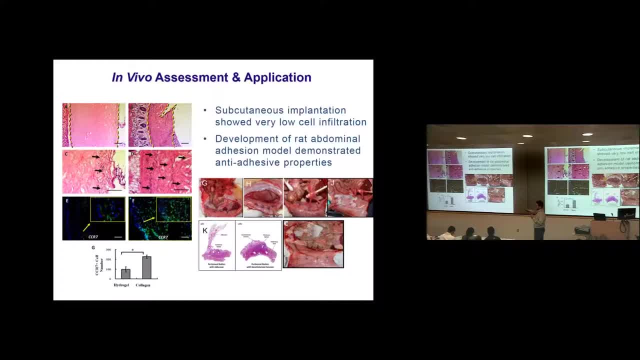 At two-week time point after transplantation you see many more cells inside that collagen hydrogel. So it's a body response. I mean it's very normal. Whatever you put in the body, the body will react to the implanted scaffold or material device. 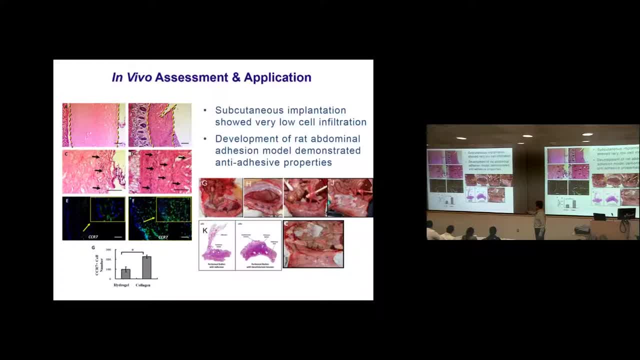 But in the amnia hydrogel actually you don't see that many cell infiltration. A lot of cells are on the surface but they cannot go very deep. So I want to do a translational research on this product. We use an anti-adhesion model in the rat model. 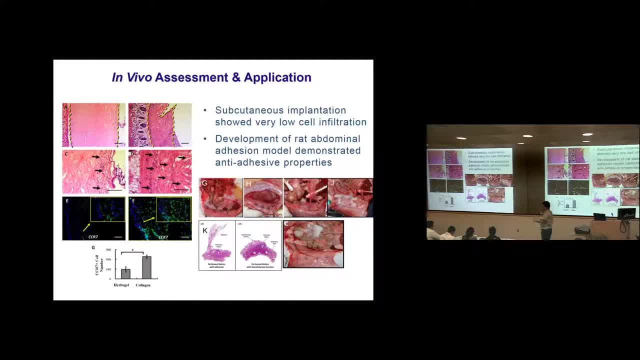 So we have two different products. One is a sheet that right after decelerization you have a sheet membrane, And the other one is an injectable hydrogel. So this is the model that we created in the lab and it's pretty well established. 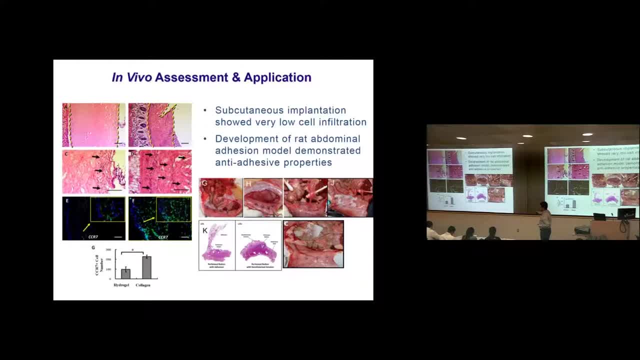 So without any treatment the abdominal adhesion will form very on all these buttons very significantly. But when you have a coverage of the amnia membrane, actually the adhesion is inhibited in the buttons that are covered by this amnia membrane, not on the other ones that are not. 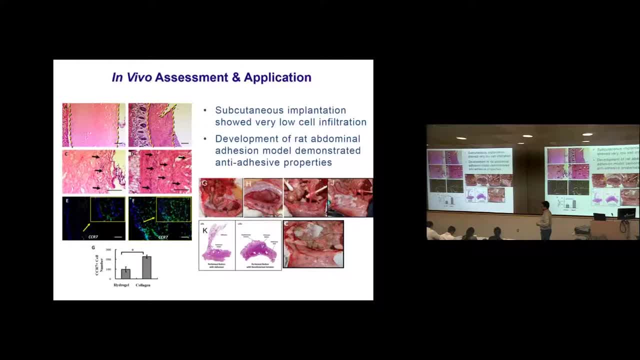 covered by the amnia membrane And injectable material is even easier for application because you can just smear it all over the place and they actually inhibit the adhesion formation quite significantly. We don't have very many animal number at this point, so we're going to repeat this experiment. 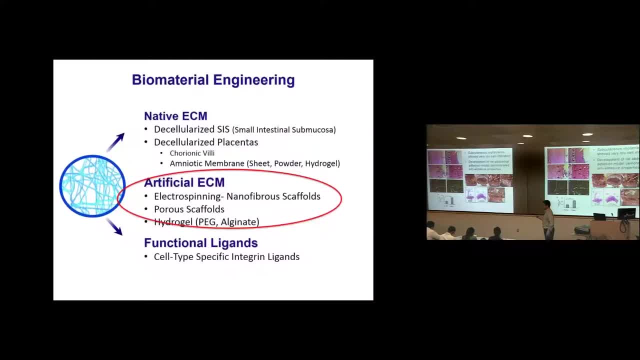 and we're going to do more, So we're going to do more research on this. I think it's a very important product, So I think I have shown this. I don't know, I have a few more minutes, but very briefly. 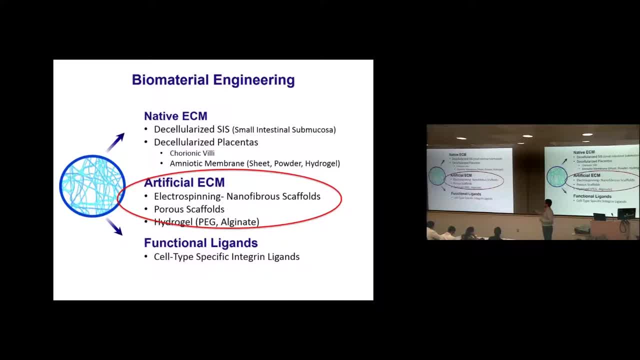 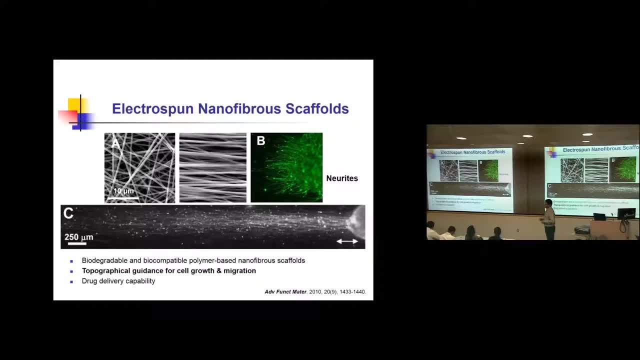 about the artificial ECM. So I want to show you what we can do in the lab, how to You can make some native ECM, but you can also engineer, make some product on your own. So one very powerful tool is the electrospinning. 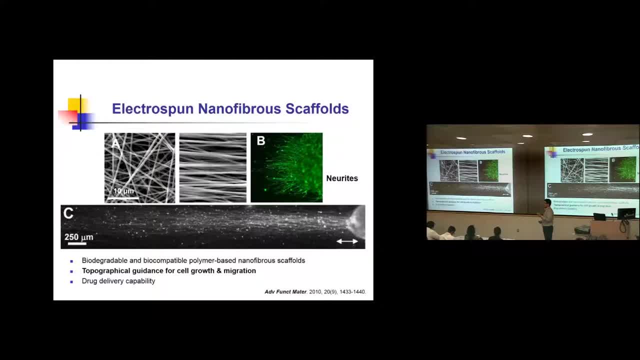 We have a machine in the lab that you can use to spin polymer into nanostructure nanofibers, for example, And you can make nanofibers align in a certain direction And the cells actually can sense the alignment. They will behave differently on the aligned nanofibers. 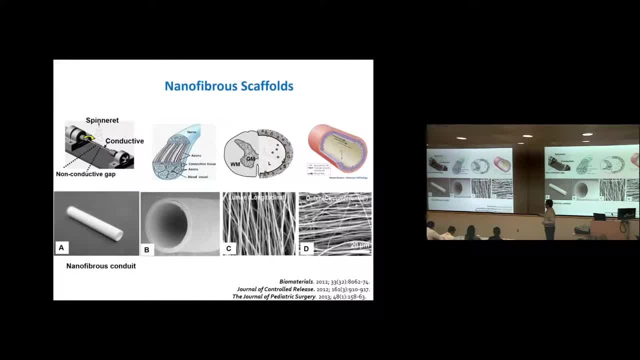 versus random nanofibers. So we can make all these nanofibers into different shapes, like conduits. You can make a line on this longitudinal line in the luminal surface, for example, and circumfinitiously align on the outside of the scaffold. 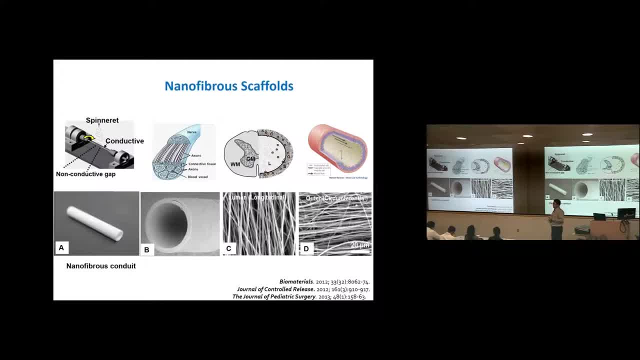 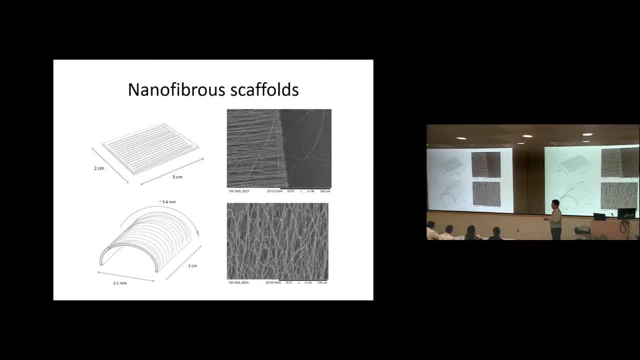 for example, for blood vessel regeneration, just to mimic the tissue that you want to replace, the tissue you want to cheat. So we've done something for the Spina bifida application, actually for spinal cord. This is done by Payam, actually quite a few years ago. 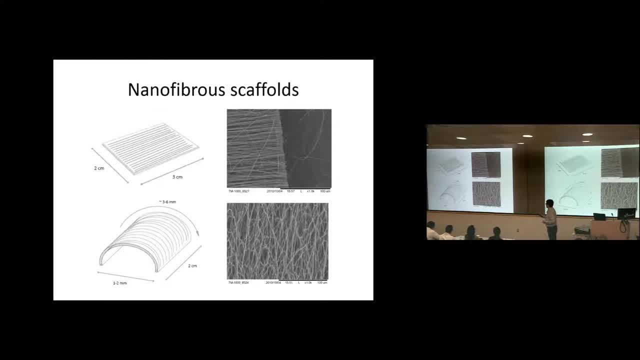 And that was still Berkeley and he was at UCSF. We can use this, the same technology, to make different shapes. So, for example, for the Spina bifida or spinal cord regeneration scaffold, you want to make the longitudinal aligned fibers in the luminal surface so that we're 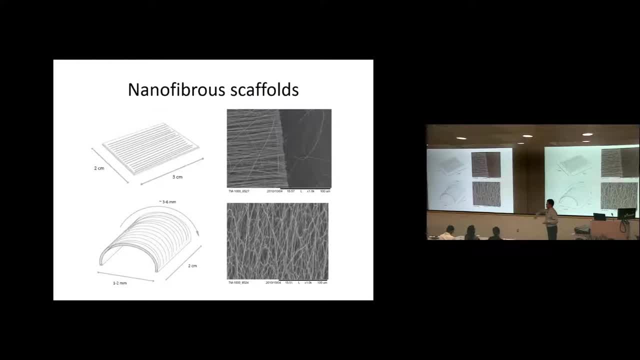 hoping the axons will grow longitudinally so that they can connect with others. So that's why we're working around more efficiently On the outside. you want to make some of this kind of directional fibers so that the suturing capability is higher, the mechanical strength is higher. 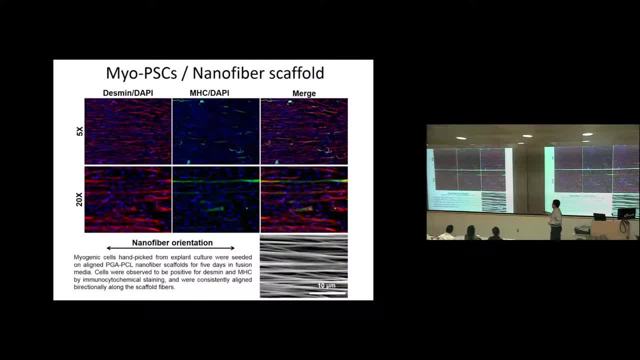 But you can make many different applications. This is a very recent data that we obtained By using these aligned nanofibers. we have myogenic cells, muscle cells. When you culture muscle cells on the aligned nanofibers, the alignment can actually help cell fusion. 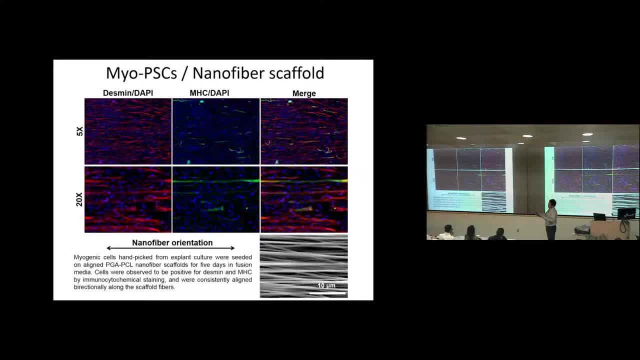 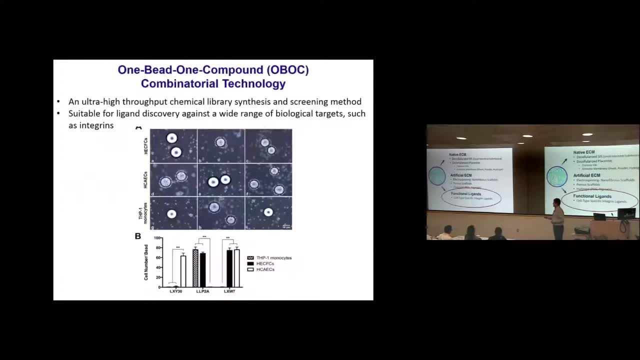 to make a more powerful cell myogenic population or muscle- cell fusion. So I'm going to skip this. This is very, very advanced actually. I wish maybe next time I will talk to you more specifically on this project. This is a high-throughput screening system. 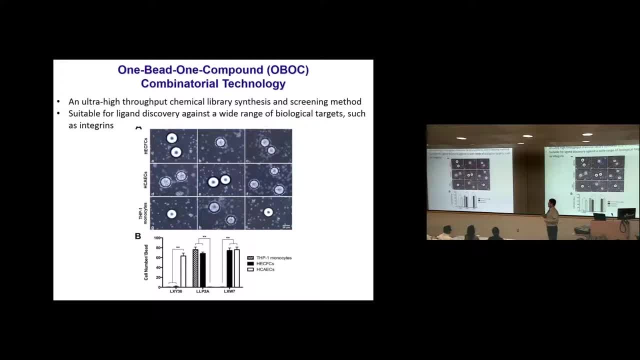 that we can use to identify specific ligands for specific cell type based on the cell surface marker, especially integrins. In this particular case, we're using endothelial cells as a model, because endothelial cells are very important for tissue regeneration, endogenesis, wound healing. 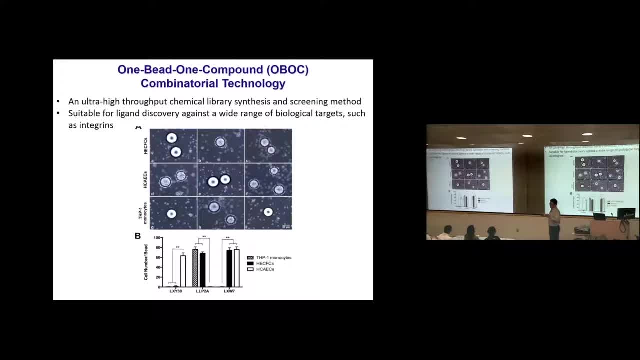 everything. So we know surface marker expression on endothelial cells or many other cell types. Then you can use 1B1 compound, the high-throughput screening technology developed by Dr Kit Lam on this campus, actually in the biochemistry department. 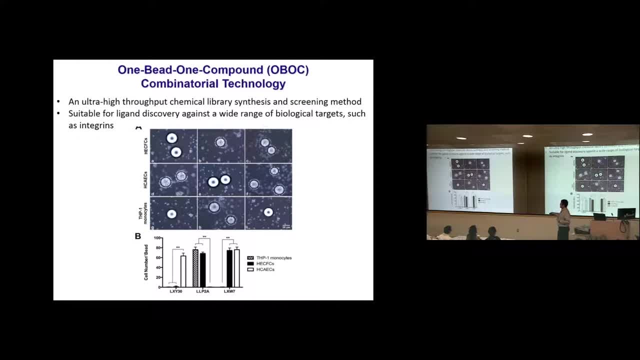 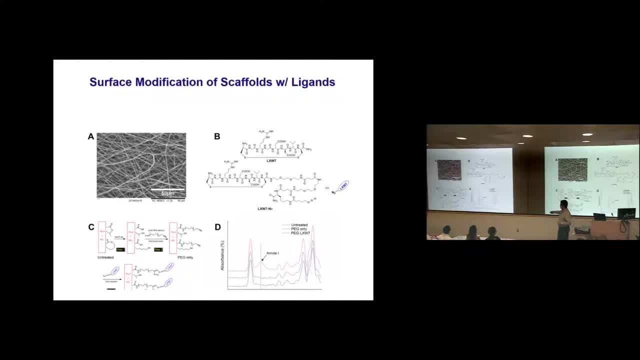 So we have been collaborating on this project for a few years Now. we've developed quite a few very powerful ligands that we can use to modify scaffold. So I won't go into here. but based on some chemistry you can present a ligand on the surface of a inert material. 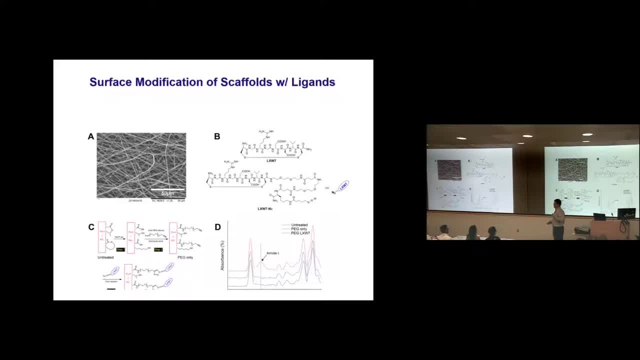 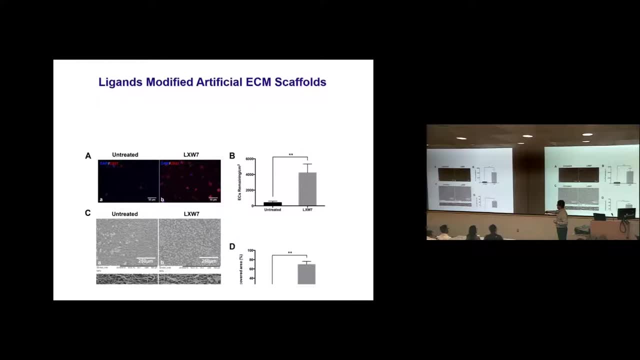 so that the inert material will become more biological active And you can design the surface, make them very in the way that you want them to be, For example, endothelial cells. with this ligand, actually, you can see much higher cell binding affinity. 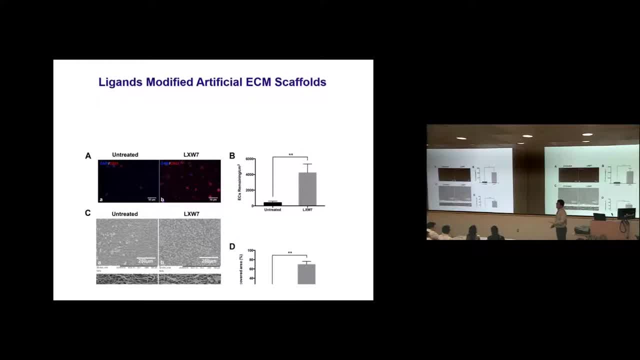 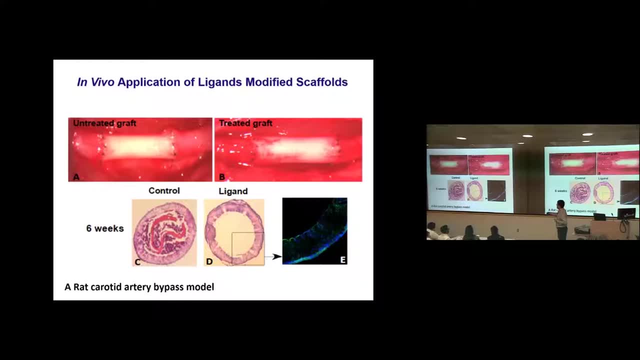 on the modified surface, compared with the inert material or the unmodified surface. This is a Evivo animal model. in the red This is a carotid artery bypass model, So you can see the ligand-modified artificial vessel graft. they are more patent. 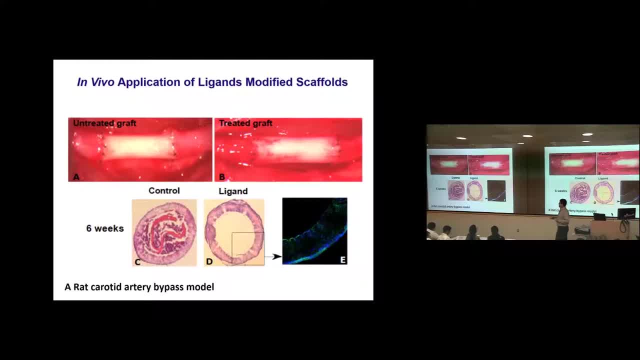 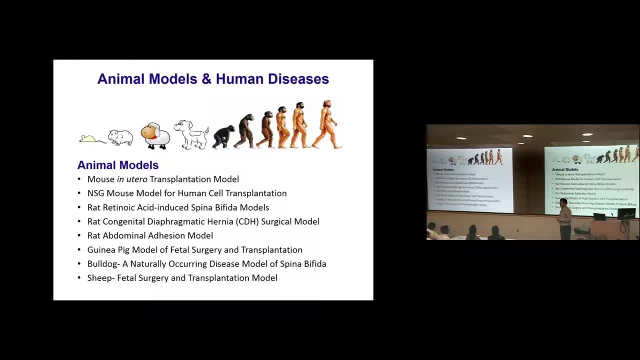 than the non-treated control vessel graft at a certain time point. So last slide, basically about animal modeling. So maybe I will talk to you more about the ligand. I think that can be very useful for many, many different projects. The ligands can be used for different cell types. 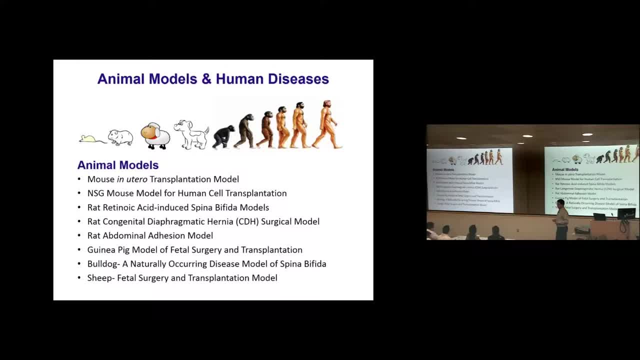 but I would have to skip that. So these are the animal models that we're using in the lab. So when you have a product, before you move into clinical trial you have to do some functional assay and Evivo animal models. functional assay: We have mouse in utero transplantation model. 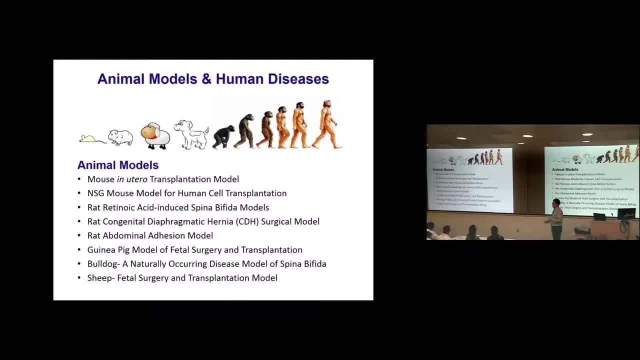 So in the mouse model you can transplant stem cells or anything that in utero before the baby mice are born, And we have the not SCID gamma, which is an immunodeficient mouse model very widely used for human stem cell transplantation And to look at the human cell. 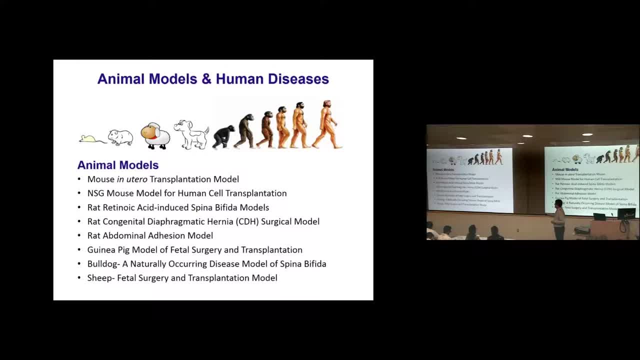 We also have a fate after transplantation. We have a rat spina bifida model, rat noic. acid-induced rat spina bifida model. We also have a rat CDH model. We have a rat abdominal adhesion model that I mentioned earlier. 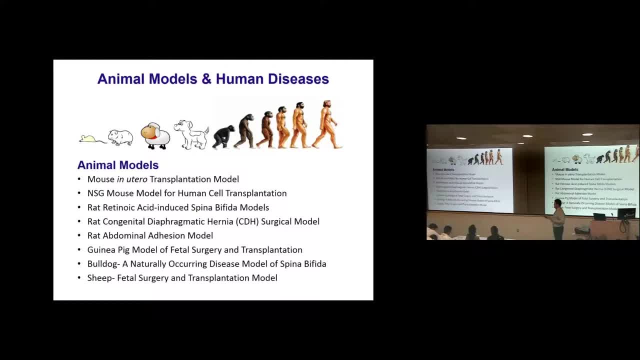 We are going to establish a guinea pig model for fetal research for many, many reasons, And we're also developing some very interesting collaborating with the vet school on developing some naturally occurring disease model. And we have the surgically induced animal model And, of course, we're still doing a lot of the sheep model. 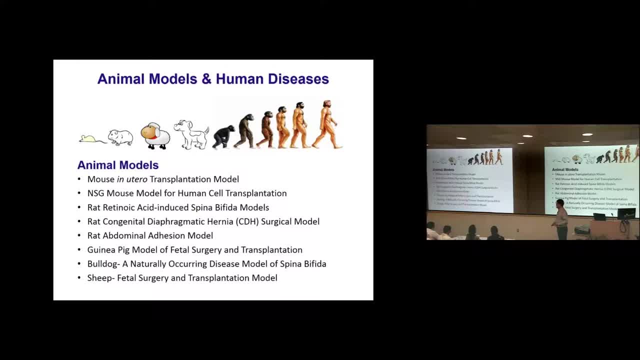 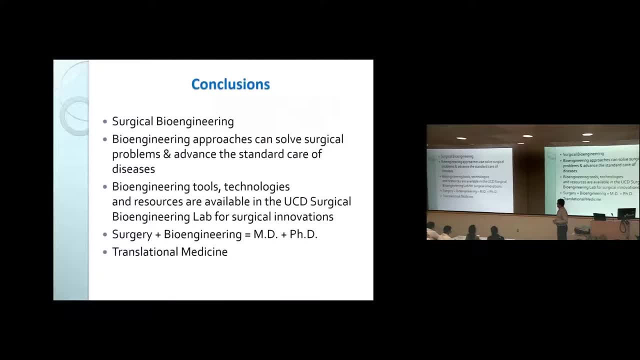 We have the pregnant sheep and spina bifida lambs And we're doing research on that. If you have any interest in any of these for your stuff, just go ahead, let me know. I think that we can help. So, in conclusion, I hope I have confused you enough today. 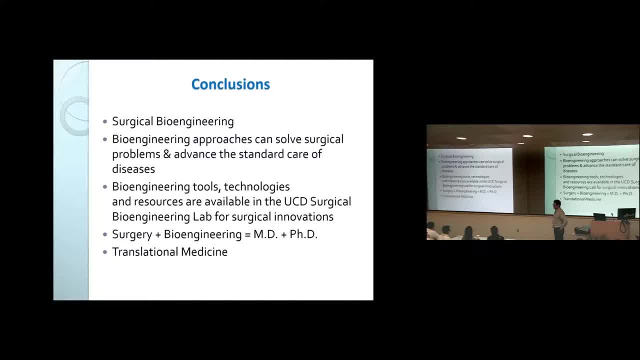 There's many different things going on. I was trying to cover- But I think I want to tell you what I understand- the surgical bi-engineering lab here at UC Davis School of Medicine. So what bi-engineering can be used for all this surgical? 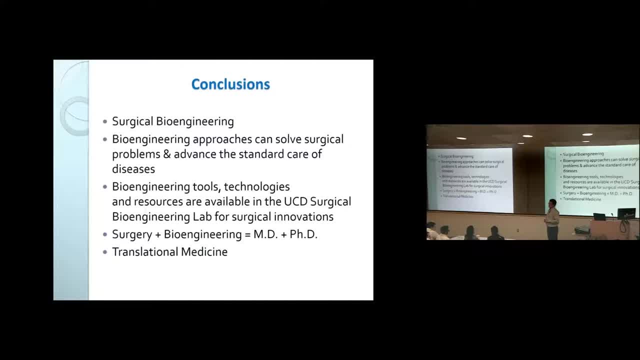 disease treatment is what we call surgical bi-engineering, All the available bi-engineering tools and technologies that can be used to improve surgical practice, to make your product better or make a new product. And also, we're hoping, and as you see, for example, 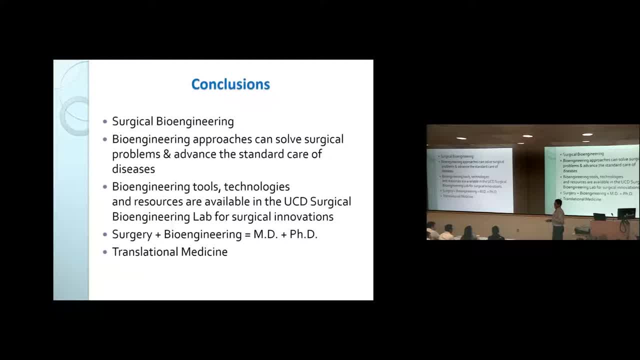 the sheep spina bifida model for fetal research, fetal treatment. The bi-engineering approaches in that particular case is ECM, cell co-culture, so that cell secretion can be monitored or can be changed. So we can use these bi-engineering approaches to improve the standard of care for many disease treatments. 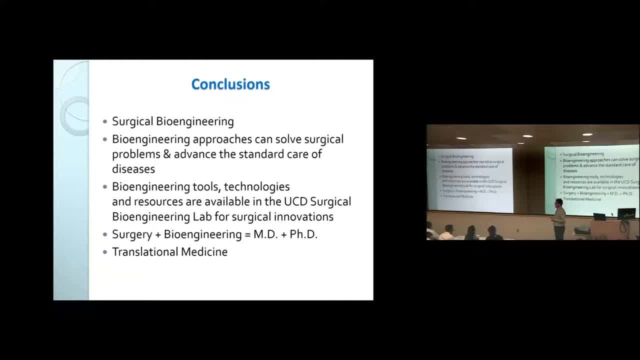 And also we have so many tools available in the lab and technologies. if you have any needs or interest in any particular thing, just go ahead, let me know. I think we're interested in doing more surgical innovations for any of your projects or interests. 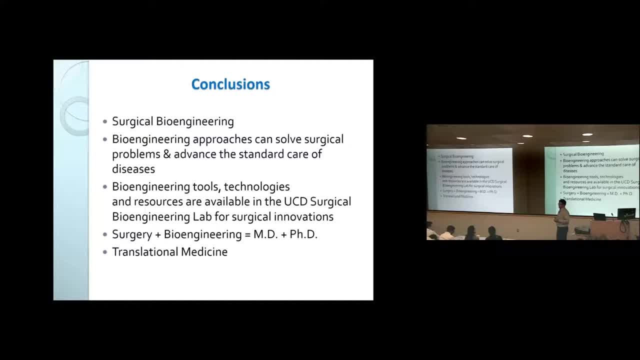 I think now we are mature enough we can provide a lot of consultation or technical support. So what we do actually in the lab is trying to just bring MDs with the PhDs or technical bi-engineers just together so that we can do our practice better in the future or now. 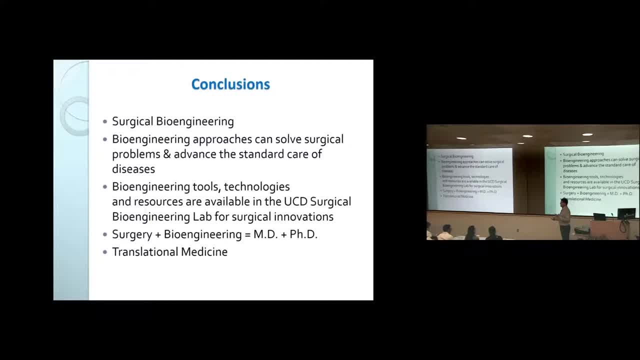 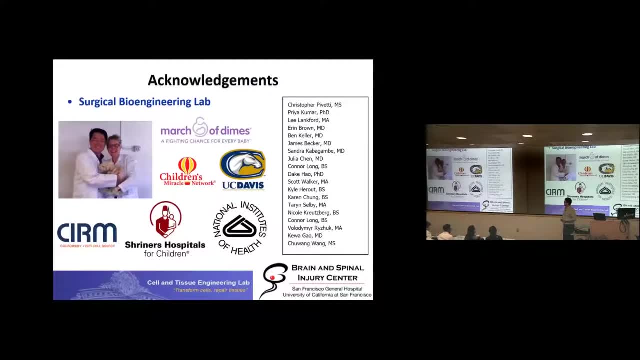 So all we do is translational medicine- Any needs that I like to talk to many of colleagues about ideas or need that you want to do, so I think our lab can potentially do something for you Dr Farmer mentioned before she left. actually she said: 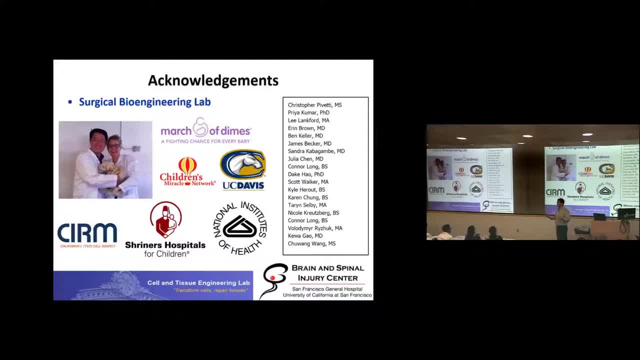 oh, you should tell everybody that bi-engineering can solve all the problems. But I think maybe one day I can really confidently say that At least now we can do something to make the change, make it better. Thank you for all the work that I presented today. 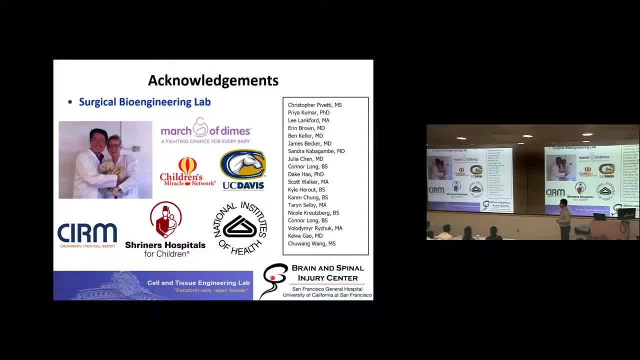 It's now done by myself, It's by a whole group of people, And we have a lot of surgical residents, We have postdocs, We have graduate students, We have project scientists, We have technicians, undergrads and many, many different. 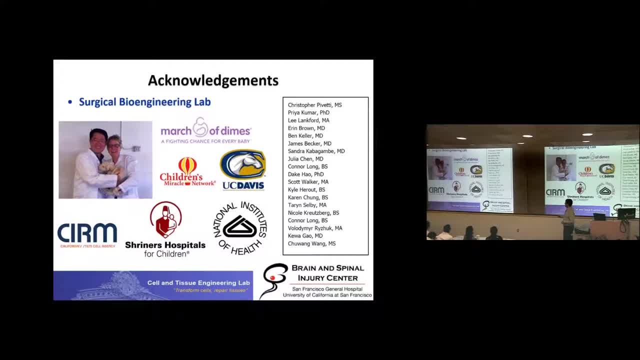 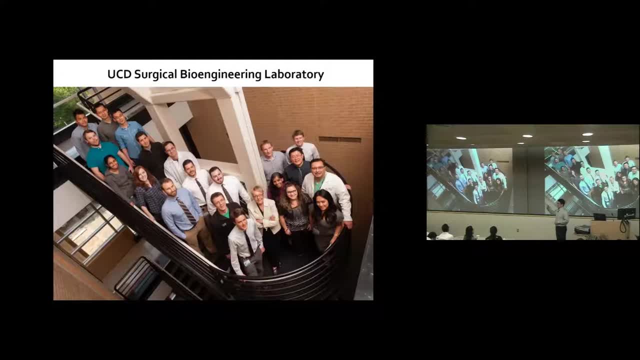 students and technician people Very appreciate all those help. We have all these fund sources And this is well. this is now the most updated picture of the surgical bi-engineering lab. We have the lab in the research two building. So if you have time, just come. 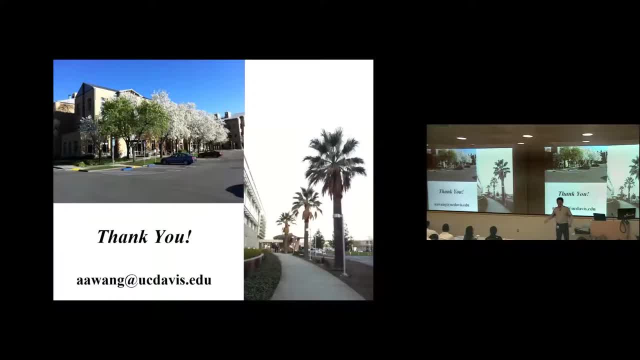 Stop by and I'm going to talk to you more about anything. This is my email. Thank you very much. Well, a tour de force summary of bi-engineering and scaffolding in stem cells. Thank you very much. How many surgery residents or fellows? 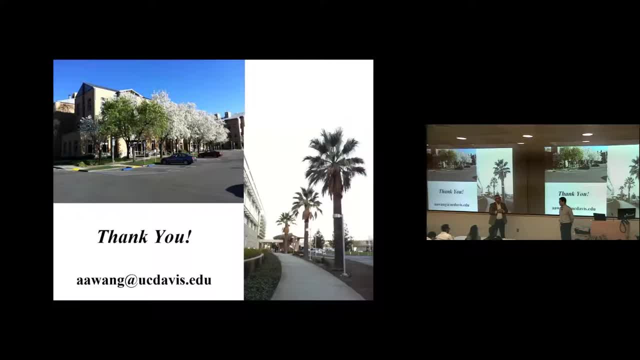 are in the lab at any one time. So at this point we have three, Three, Yeah, usually two to three, Yeah, Yeah, different years. And again, thank you. Any medical students, undergrads students? Yeah, so I have trained many. 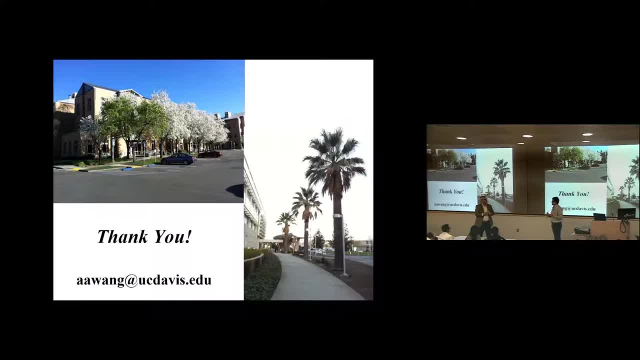 Well, we have many pre-med students who are interested in applying for med school. They want to get some research experience. We also have trained some medical school students, summer research time projects, those kind of things. Any questions, Dr Brown? 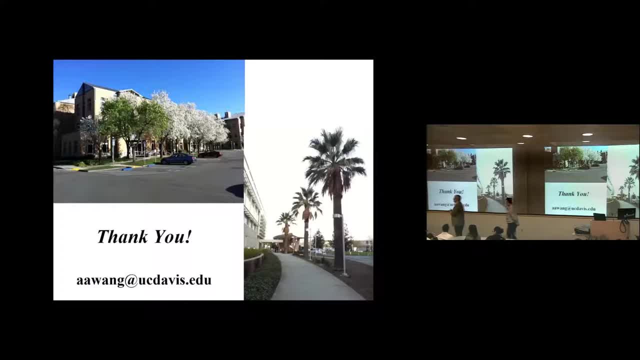 Yeah. so with the stem cell approach the challenge is always getting approval because of the risk of cancer Right, the potential success of paracrine or the supratone aspect of it. Is there any concern that the supratone changes? 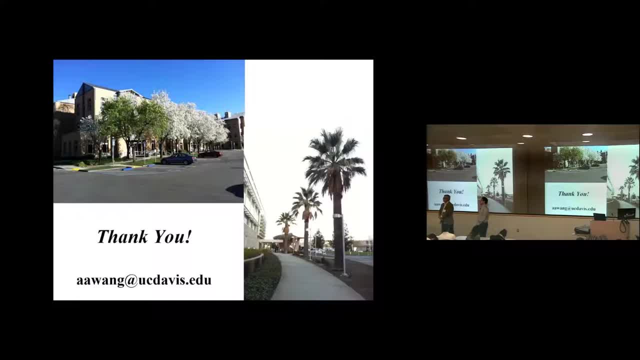 in the context of being in vivo? And if so, are you able to perhaps recover your matrix over the first two weeks of placement and then chromatograph it essentially get a separation of what that supratone looks like Over that two-week period, because that would give you 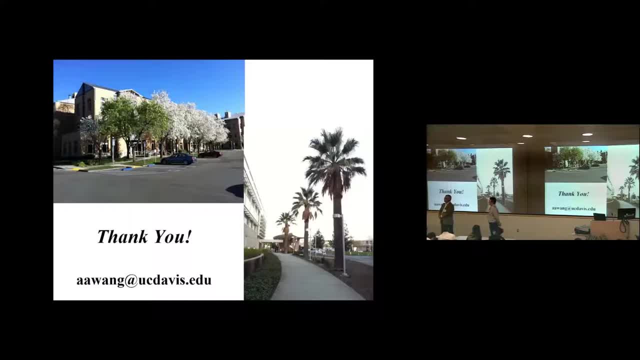 potentially the complete cell-free package that. you were Right, That's a fantastic idea So well as you mentioned. very true, that stem cell product is very great, but you have to go through FDA approval- very tedious. You need to have a GMP facility to get this live cell product. 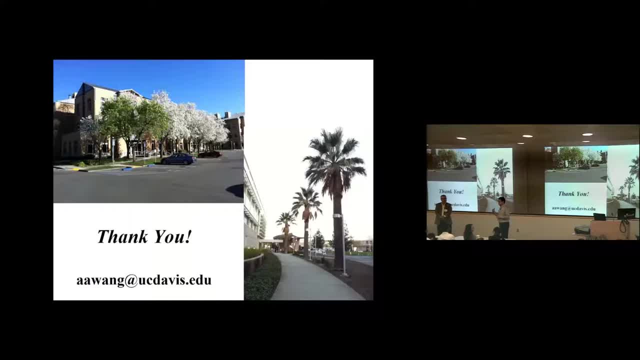 and there are many safety issues with that. So what we're trying to do, what we're doing- stem cell product very actively now, but on the side- the other side- we really want to develop some cell product, a cell-free product, so that can hopefully mimic the cell product. 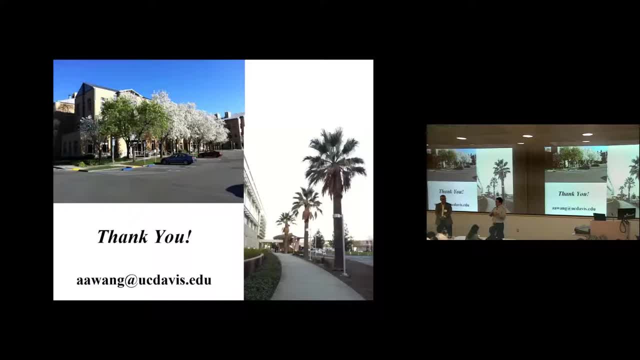 As you mentioned, very true that after you transplant live cells in vivo at different time point, the cells are changing. They are changing. I think they are really changing especially, I mean they die off over time. They must be changing significantly. 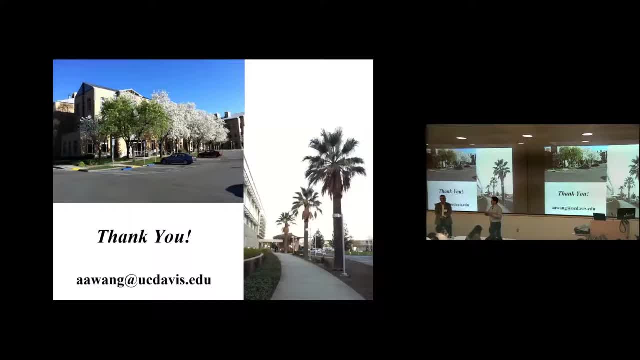 So we cannot really control the cell fate once you inject or transplant the cells in vivo. but I think if we really want to want to develop a cell-free product, we can If you want to develop a accurate mimicking for the live cells. 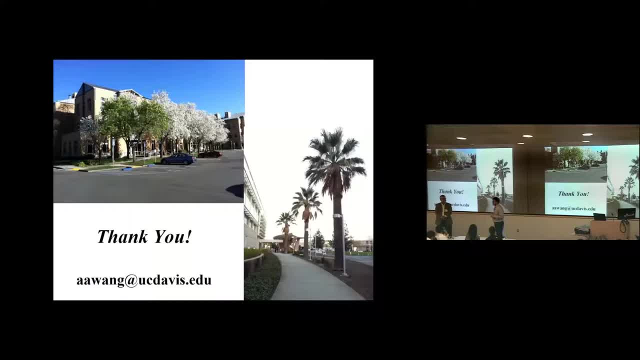 you would have to go in there and look at different time points, probably Exactly. That would be great, but I think that's doable because the injectable or infusionable exosomes, for example- they are just like a drug. 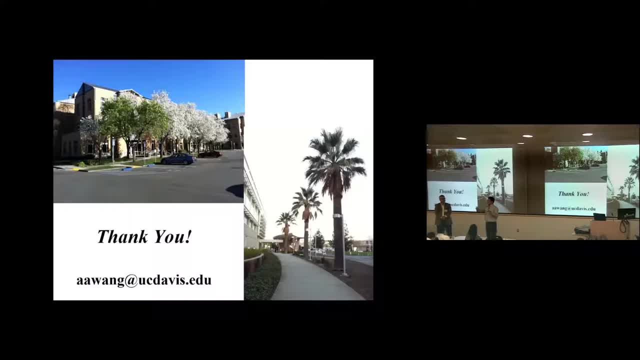 You can inject at different time points, right? If you know how the live cells are behaving in vivo at different time points, you direct that product properly and you inject them during that. That would be a very fantastic approach. Scott, are you worried about retroviral contamination? 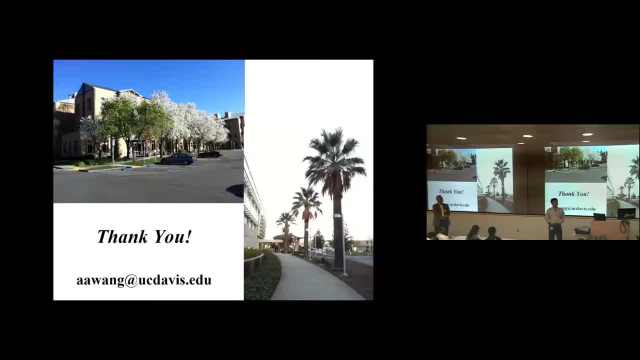 of the exosomes And if so, what are you doing to mitigate against it? Yeah, well, that's a great question. So as far as I know, in the US right now actually there's no FDA-approved product yet. 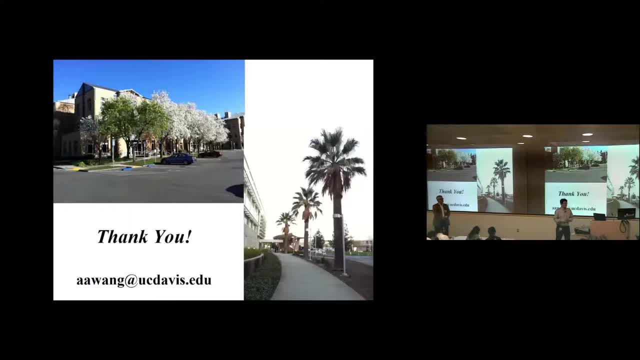 But in Europe actually they have some clinical trial going on already about this, But so far there I haven't seen very, very significant adverse side effects of the exosomes for the viral contamination or anything. But I think that's certainly a very important thing. 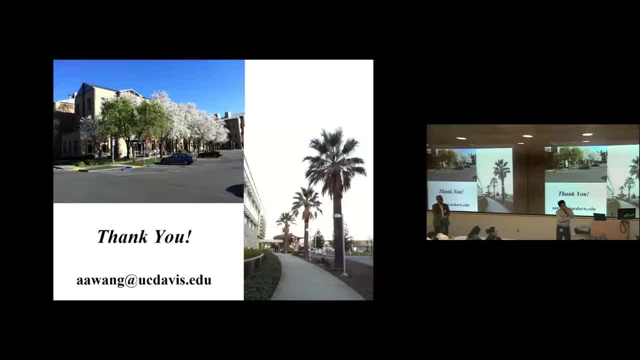 to look at. Is there some sort of primitive screen for retroviral Right? Yeah, I haven't seen any publication. actually, This is a very new field. Exosomes have been described for many years, but for regenerative medicine application. 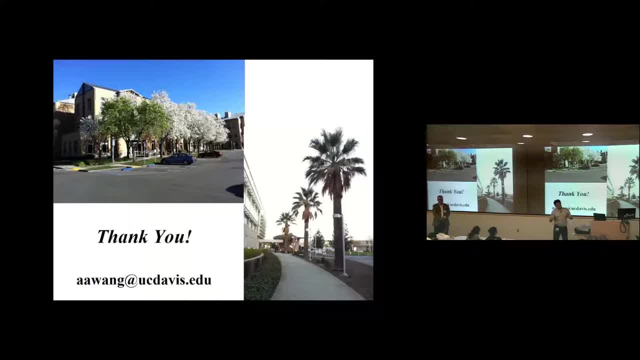 just a few years old, But now actually Many people are in this field and trying to develop this as a product. But I think many things need to be learned before we can really translate Black boy. Excellent, Thank you. According to bioengineering, the role is no question. 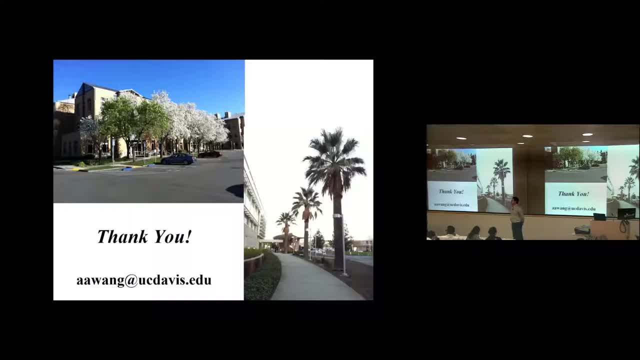 of, And there's so much in your presentation. I was going to point this in one very small aspect, That is, you need to know your thoughts on the role of the age in the ECM, on how it affects your actions. Yeah, 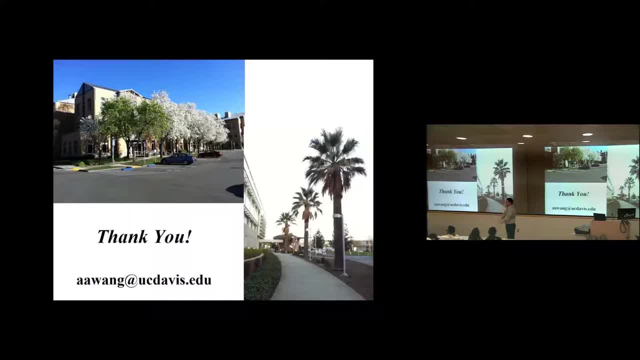 Right, Right, Yes, Yes, Right, Right, Right. The youngest matrix. The matrix is a 3D construction and you start chomping it down. 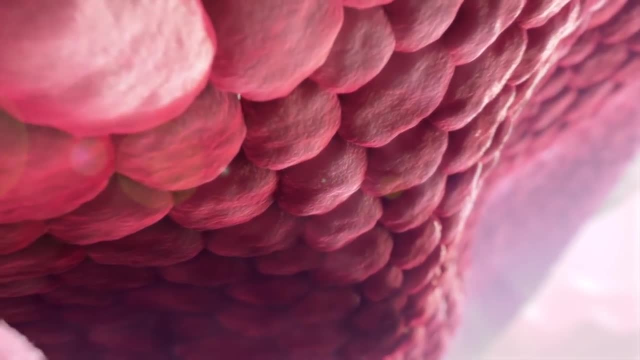 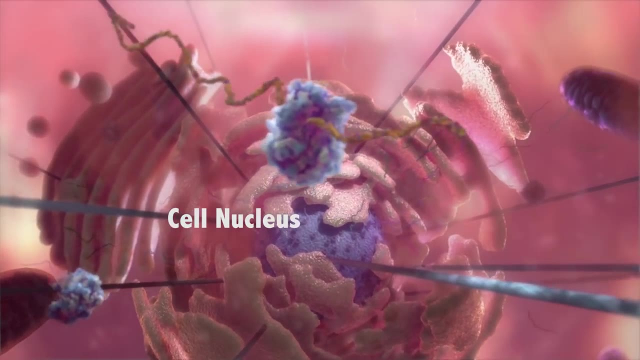 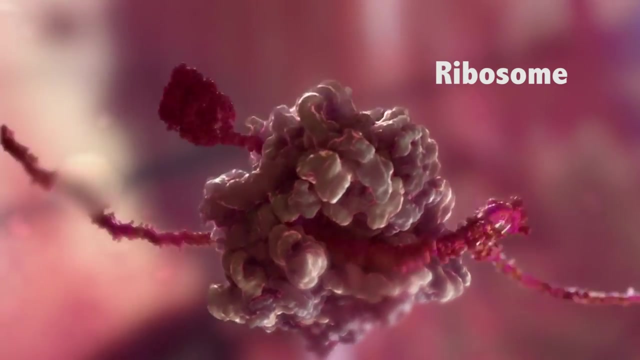 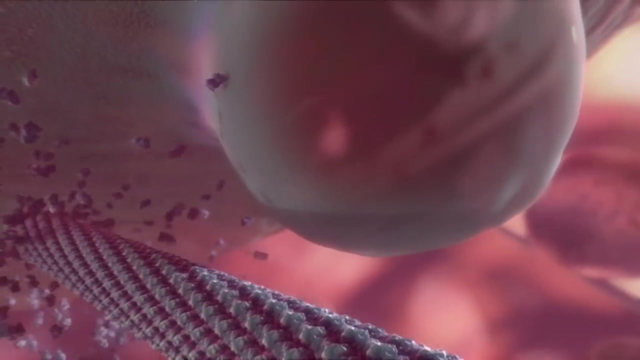 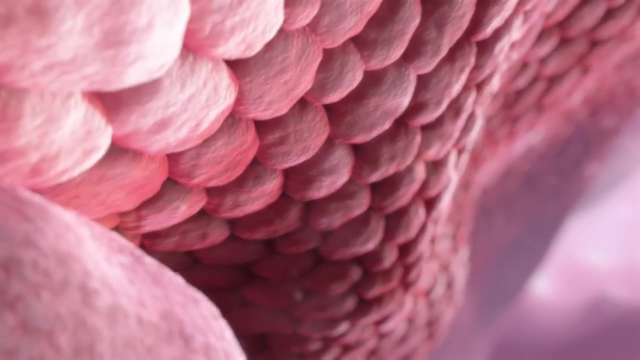 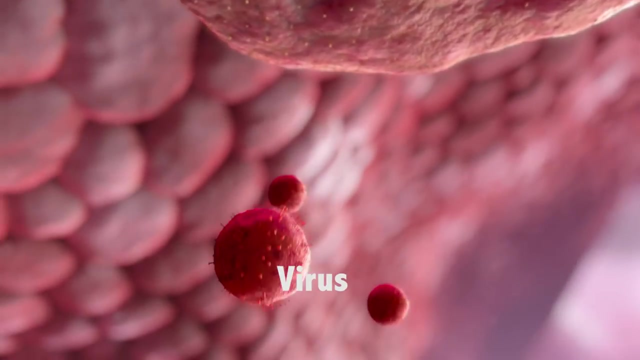 Every cell in your body is a tiny factory constantly making proteins. Your genetic code, or DNA, directs every activity. Protein-making machinery in the cell reads the cell's own DNA and makes sure the cell proteins go where they're needed. Viruses have their own genetic code, but they don't have the machinery to copy their DNA, So 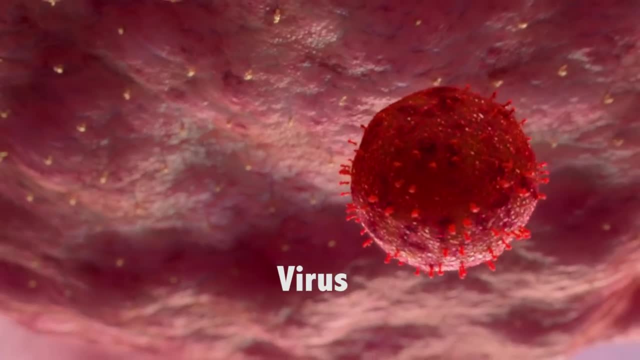 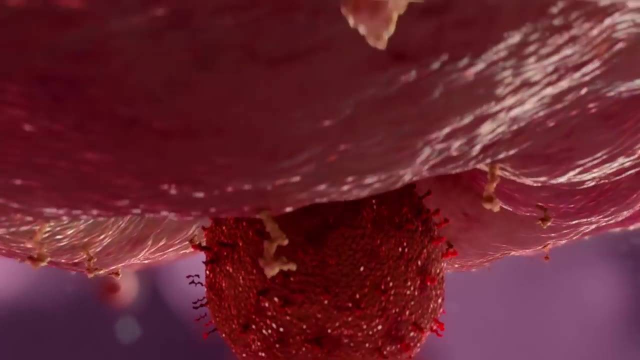 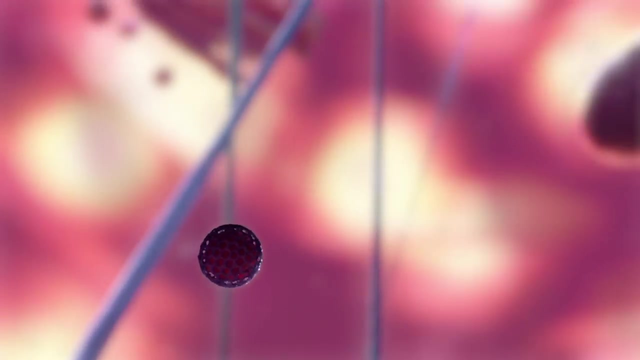 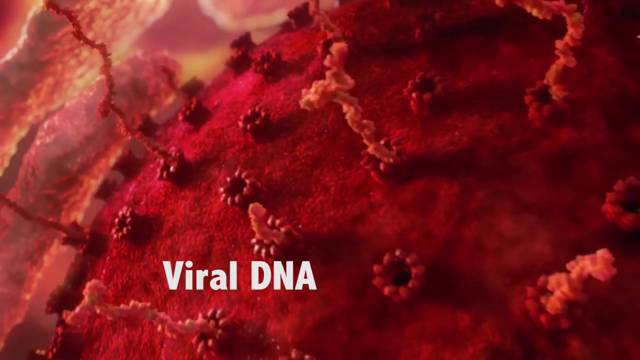 viruses need your cell's machinery to reproduce themselves. A virus starts this process by using the keys on its surface to gain entry. Like a Trojan horse, it enters the cell. The virus releases its own DNA into the unsuspecting cell and hijacks the protein-making machinery. 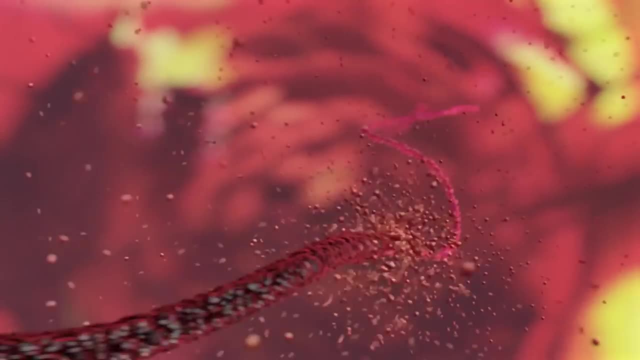 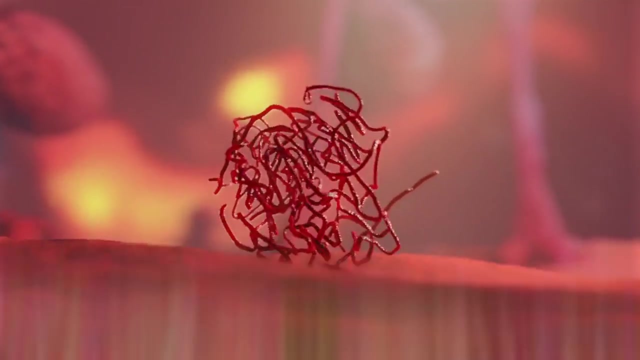 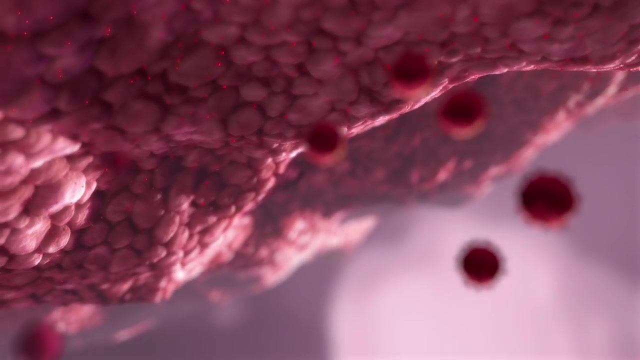 Now this vital cell function becomes an assembly line for new virus particles. No longer in service to your body, the cell now serves the virus, manufacturing thousands of new virus particles which are released to enslave more cells—thousands more cells.